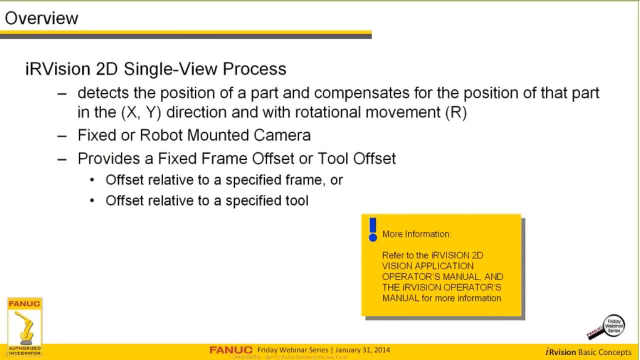 And please feel free to ask questions as we move along. So the IR vision 2D single view process: what does it do? Well, the IR vision 2D single view process allows you to see the position of a part and provide the compensation to the robot program for the position of that part in an XY direction and with rotational movement. 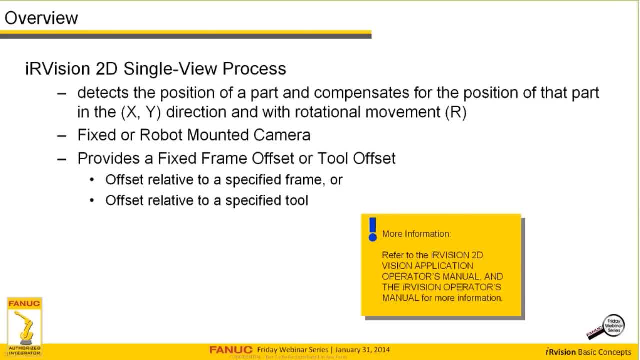 2D imaging does not provide a Z-axis height, nor does it provide any information on yawn pitch. We presume, when we're using a 2D single view process, that for the most part, our parts are in a planar representation perpendicular to the camera and will generally only be in a single plane of view. 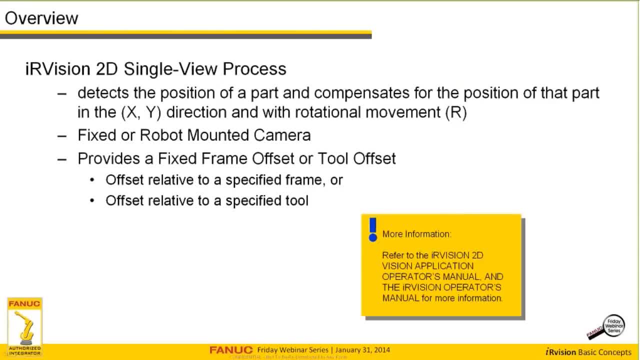 The 2D single view process can use either fixed or robot mounted camera, And for our brief tutorial, we're going to concentrate on the fixed camera. but all the information we provide today can be applied further to the robot mounted camera. And what does the single view vision process provide? 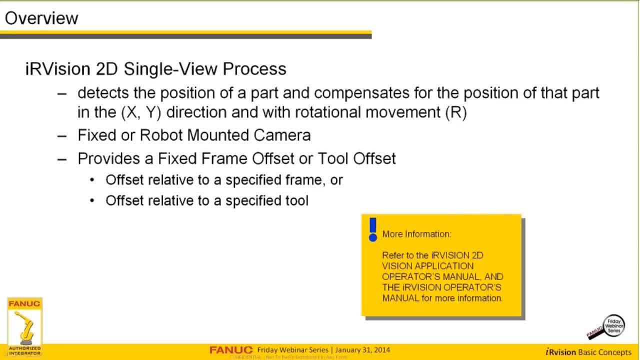 It provides either a fixed frame offset or a tool offset. Those offsets are relative, in the first case, to a specified frame- a user frame that you've correctly taught- or an offset relative to a specified tool- Again a U-tool that has been correctly taught. 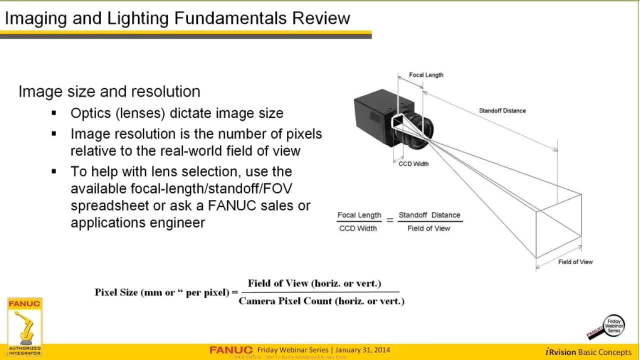 Let's talk about, briefly, imaging and lighting. Of course, this topic could be a topic for an entire webinar series, but I'll just touch upon some of the basics that you have to remember And things that I get asked frequently with respect to image size and resolution. 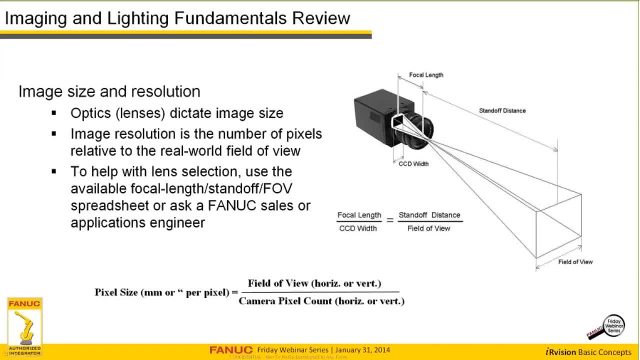 Recall that optics or the lenses are what dictate the image size. The image resolution, on the other hand, is the number of pixels relative to the real world field of view. Let's look at our image over to the side, where we see the four features, the four mathematical features of an optical chain in a camera. 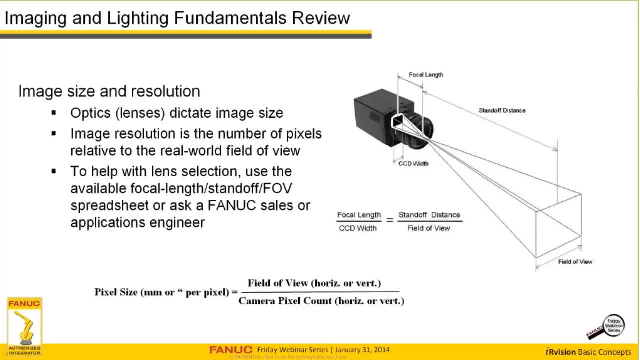 We have the width of the sensor, which is the CCD width. We have the focal length of the lens, specified by the F number on the lens. We have the standoff distance of the lens. That's also called the working distance, the distance from the face of the lens to the part of the features that we're trying to image. 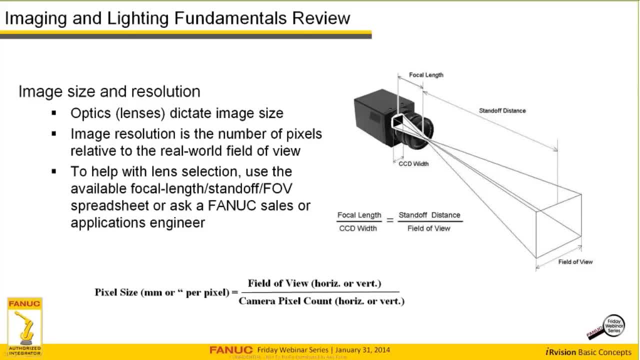 And then we have the size of the field of view. As you can see from the short, the small mathematical formula, by that image there is a proportional relationship between focal length and CCD width, as it relates to standoff distance and field of view. In short, if you know any of those three numbers, you can calculate the other number. 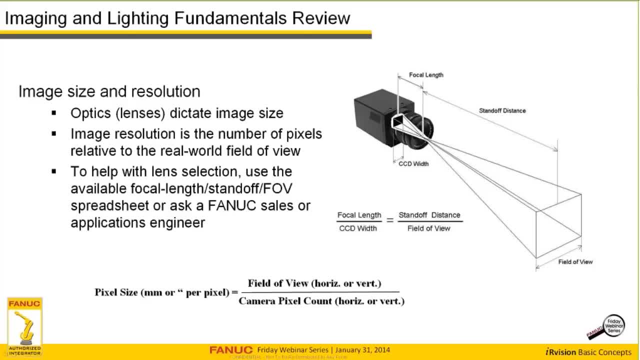 Normally we know what the CCD width is and we know whether we'd like a particular standoff distance or a particular field of view. From there we can calculate exactly the focal length of the lens we will need or the resulting standoff distance of field of view with a focal length. 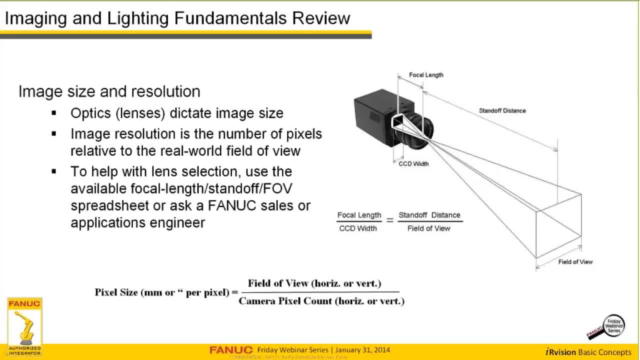 When it comes to resolution, I have another calculation down at the bottom and this is even more simple. but I'm asked often: how does the lens, the camera, the standoff relate to the resolution? Well, resolution is very simple in its concept. 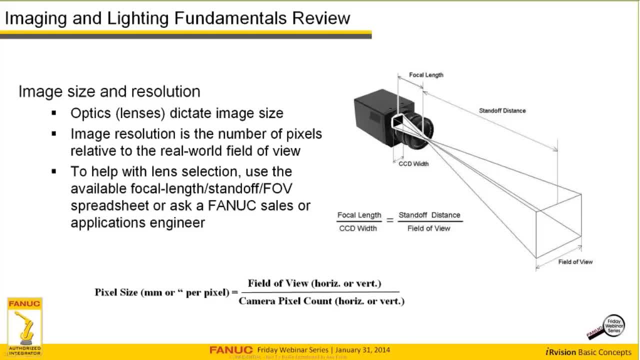 There's a pixel size related to the field of view and the camera pixel count. So pixel size in millimeters or inches per pixel equals the field of view of the overall image in resolution. So in real world, in real world measurements, either horizontal or vertical. 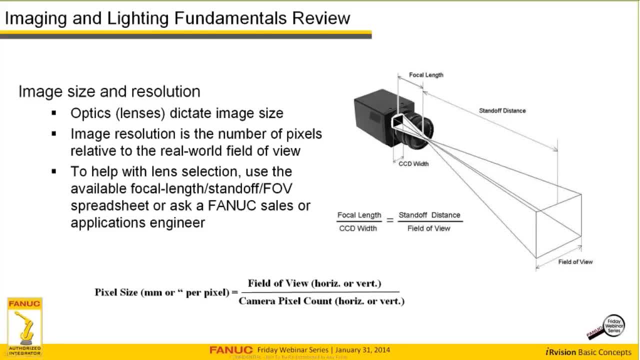 over or divided by the camera. pixel count either in the related horizontal or vertical direction. This gives you an idea of the pixel size or some people might even say the pixel resolution or accuracy in real world that the camera is able to achieve. You'll note that changing optics doesn't necessarily change the pixel size. 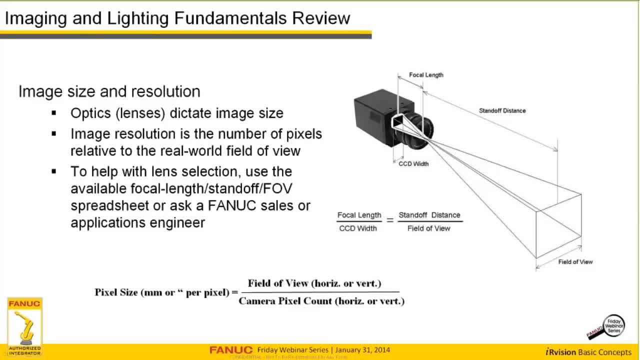 The only thing that will change the pixel size is a change of the field of view, as you can see from the calculation or the change of the camera pixel count. To help with lens selection, use some tools that are available to you. There are focal length, standoff, field of view spreadsheets available. 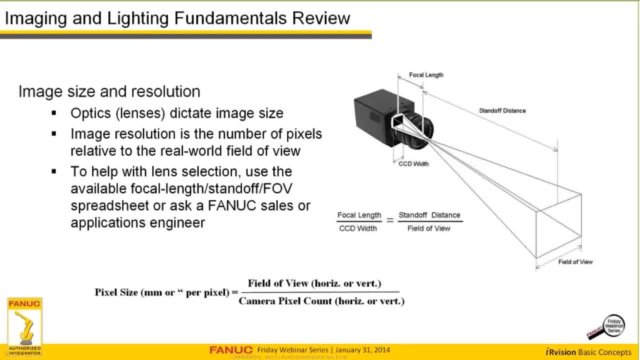 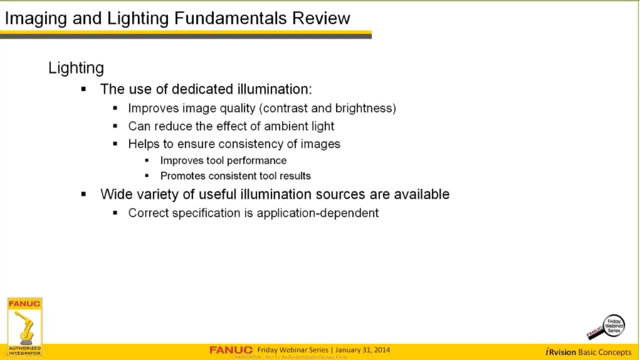 or ask a FANUC sales or application in your course. When it comes to lighting, I think you should do what we do here at FANUC with all of our demos, and that is to use dedicated illumination for your application. Use of dedicated illumination can help in a variety of ways. 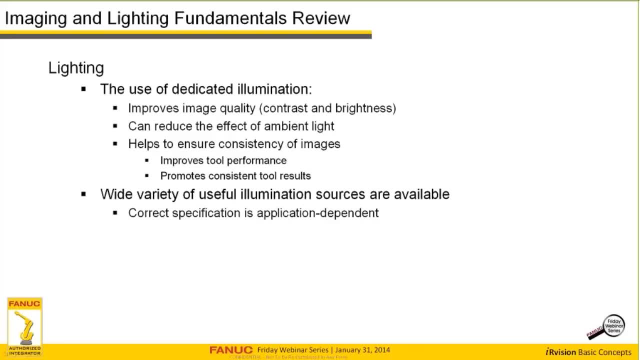 It improves image quality, and by image quality I mean contrast and brightness. We want the image to be bright enough to extract the required edges or information that we need in our IR vision tools. And when I say contrast, let's be very clear. 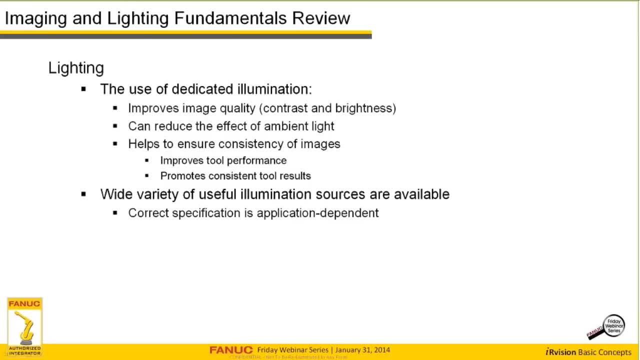 I'm talking about contrast in the sense of signal-to-noise. That means we want to make sure that the lighting enhances the image to the point where we see the best ratio of foreground- that being the part that we want to image- versus the background. 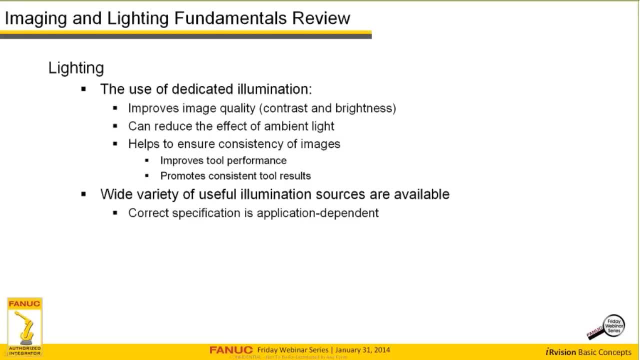 We want to highlight the part of interest and low light or ignore the background. that may be confusing. Dedicated illumination can also reduce the effect of ambient light. One of the dreaded things in a plant floor is to have a light overhead, or sunlight overhead even worse. 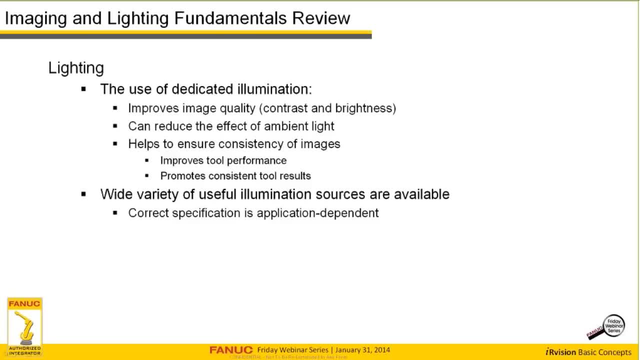 that will make your imaging inconsistent. So we want to make sure that your imaging is consistent over time and over part by part. Dedicated illumination, if it's bright enough and perhaps even of the correct color, can help reduce the effect of that ambient light. 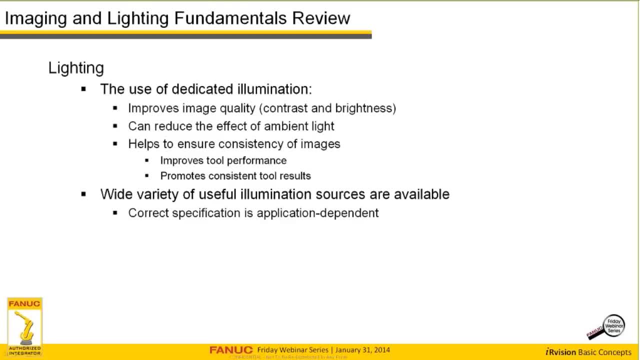 And finally, it helps to ensure the consistency of images We make part after part after part. These parts change, The positioning changes. What we want to do is have dedicated illumination that will keep that image consistent over time and that helps improve tool performance. 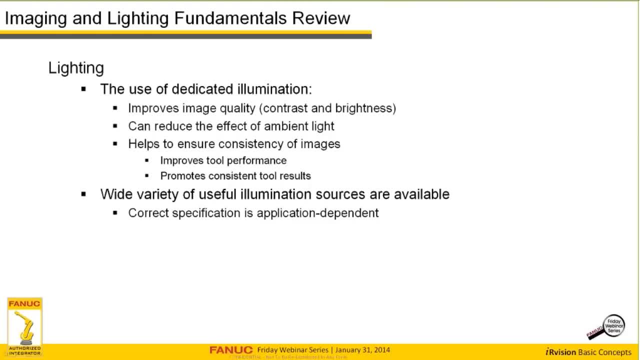 And that's gaining accuracy. overall, There are a wide variety of useful illumination sources available. There's no one rule of thumb, however, to tell you what's going to work for your specific application. It's application dependent and I highly recommend that you experiment or test lighting sources. 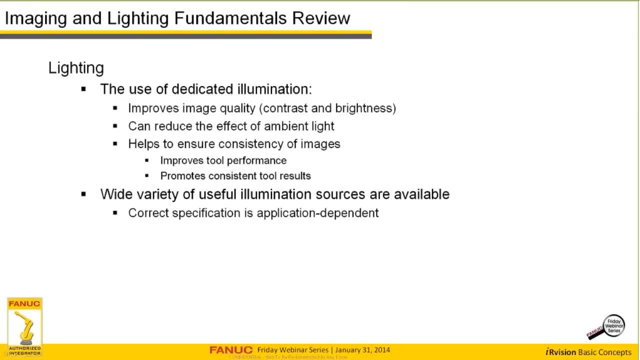 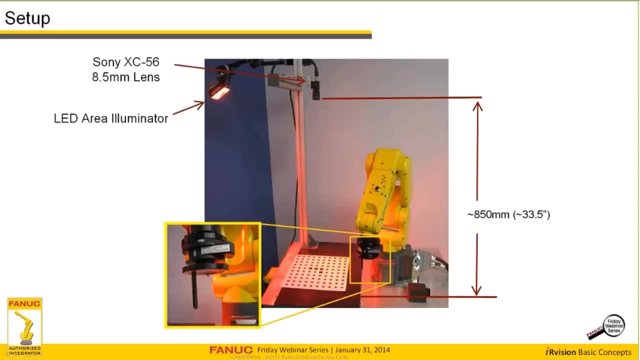 to see that you get the optimal light for your application. So, having said that, here's our setup here in the FANUC conference room as we move forward in our work. I'm working with a Sony XC56, which is the standard resolution FANUC camera. 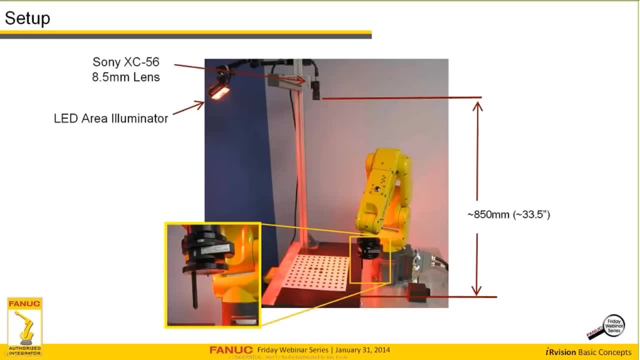 using an 8.5 millimeter lens to achieve the field of view that I want. at the standoff of about 850 millimeters, I've set up a kind of a broad area LED illuminator. Again, this is not to suggest that this is optimal for your application. 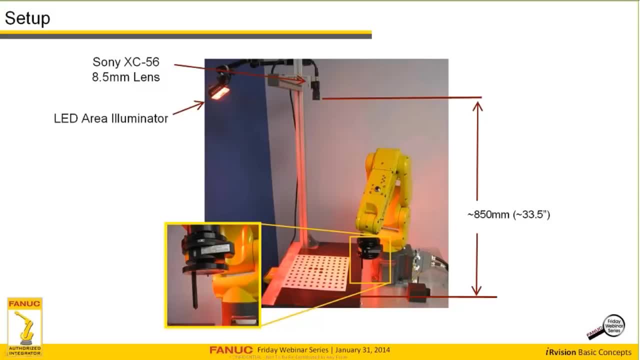 but it's going to work for our demo. I want to note that we're using a LRMate 200 ID 4S for our demo, and those of you who are familiar with this might note that it has a force sensor, an FS15IA force sensor, on the end. 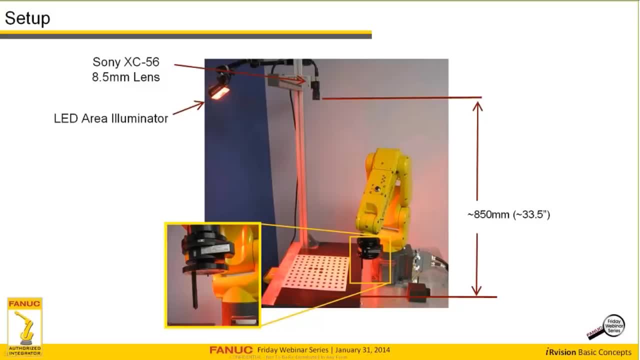 I'll point out, however, that we're not using that as part of the demo, but that's a good tool to keep in mind for your applications as well. One other thing I want to say is that we are doing this live. We have the robot and the cell, the test bed, right here beside me in the conference room. 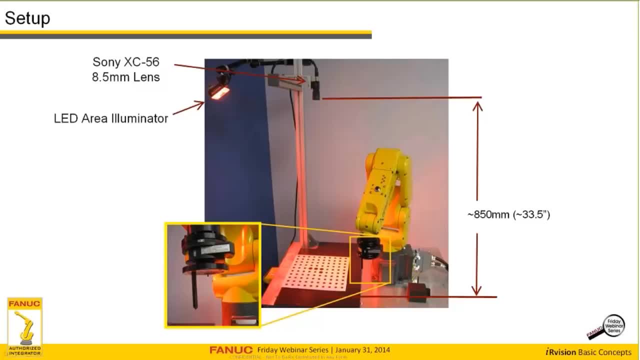 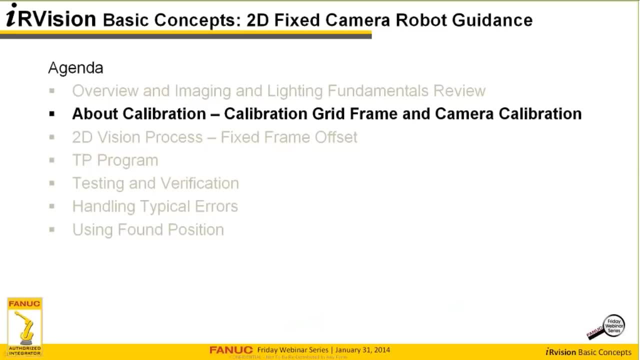 and we will be doing a good portion of this demonstration in live mode with the actual robot and actual imaging. So, with that being said, let's move on to talk about calibration, And that takes two steps: the manipulation of a calibration grid frame and the ultimate camera calibration. 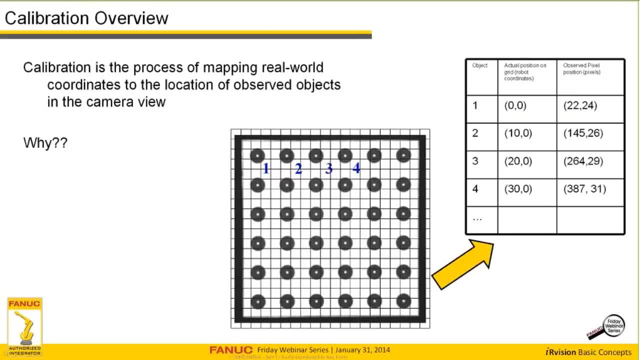 What is calibration and why do we do it? It's the process of mapping real-world coordinates to the location of the observed objects in real time. So what we're doing is we're mapping real-world coordinates in the camera view. Think about it as we look at this grid in the center. 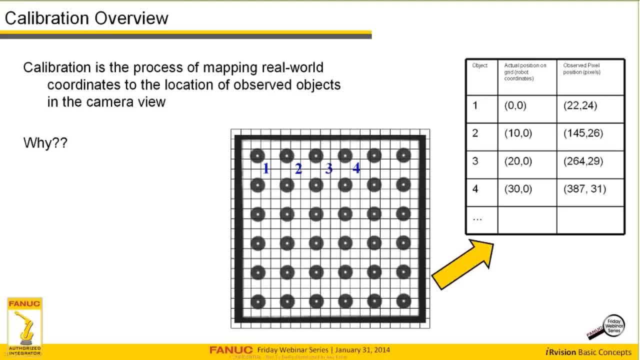 and the related table. over to the right-hand side, The calibration plate has a series of dots on it and those are known. those are actually very precise dots in real-world coordinates- known real-world coordinates relative to some point on the calibration plate. 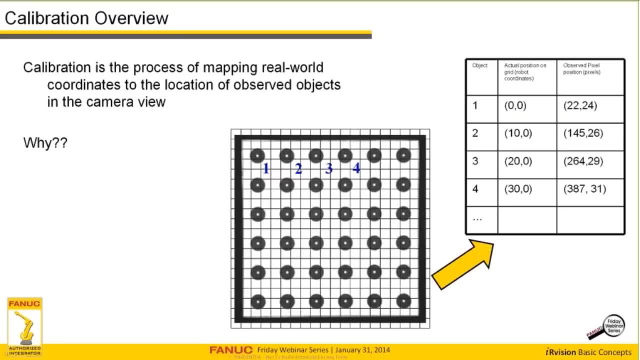 I've overlaid that And you can see that the camera view is represented by these pixels And these pixels will be the camera view. Of course there will be many more pixels, but those pixels represent the camera view of those dots. When we transform the real-world dots to the pixel space, 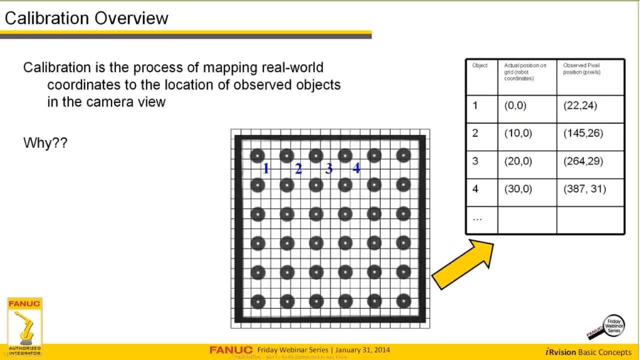 we get a table like you see on the right, where for each dot object there's an actual coordinate grid position in robot coordinates and there's an observed pixel position from the camera information. So we can see the relationship between real-world and pixel coordinates. 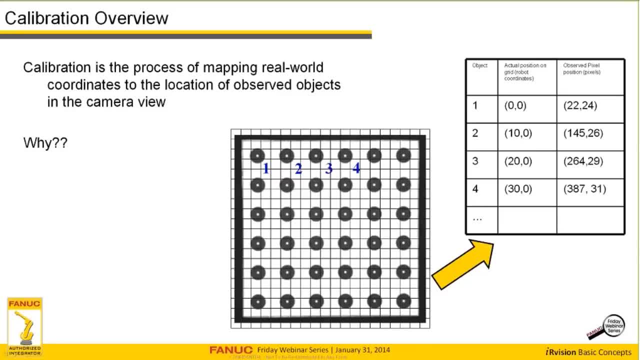 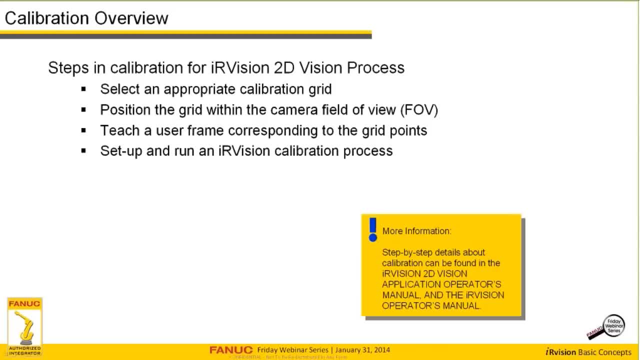 so that we can use that mapping later on to find a part anywhere in that field of view and accurately return the correct robot coordinate. What are the steps in calibration for the IR Vision 2D vision process? We select an appropriate calibration grid. We want the calibration grid to cover most of the field of view. 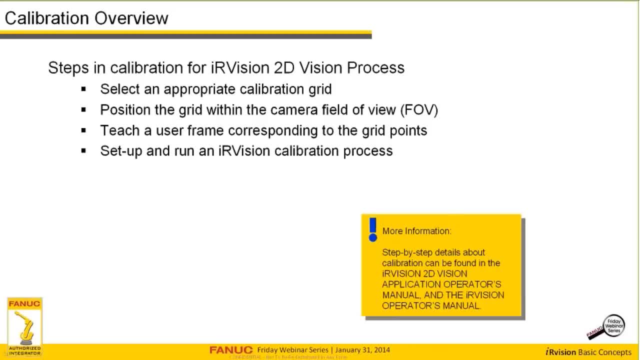 and even if it covers all of the field of view, that can work out too. If it's not covering all of the field of view, however, the areas that are not covered have to be considered as indeterminately calibrated. They'll certainly return a real-world point. 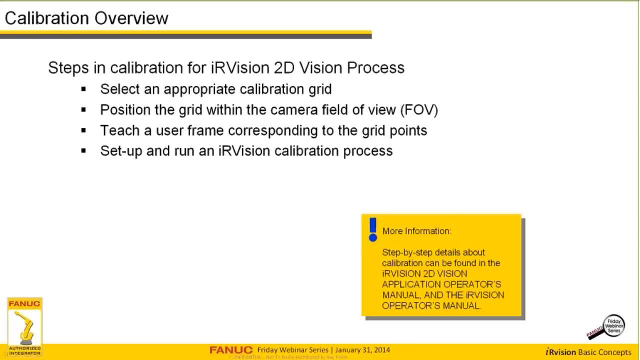 but we can't guarantee through the process that those points are correctly determined. We position the grid in the field of view As we do the grid calibration. we can later see the grid in the field of view and then teach a user frame corresponding to grid points. 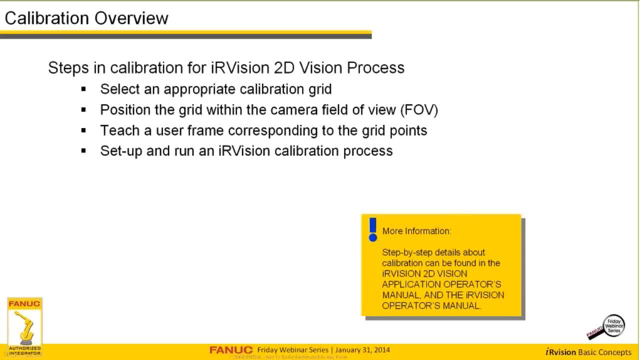 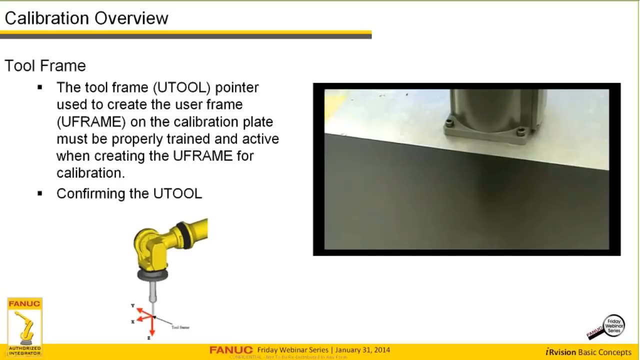 Again, I'm not going to go into a great deal on teaching a user frame, but I advise you to look in your documentation if you're not familiar with that process And then finally set up and run an IR Vision calibration process. The first step in creating a user frame is to make sure that we have a tool frame pointer. 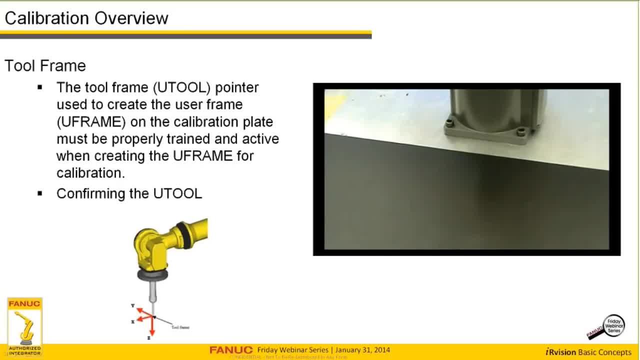 when we're doing a manual U-frame teach that is properly trained and active. when creating the U-frame, How do we make sure that our pointer is correctly trained and the tool frame is correctly trained for that pointer? I like to confirm that the U-tool is correct by placing it to a point at a known location. 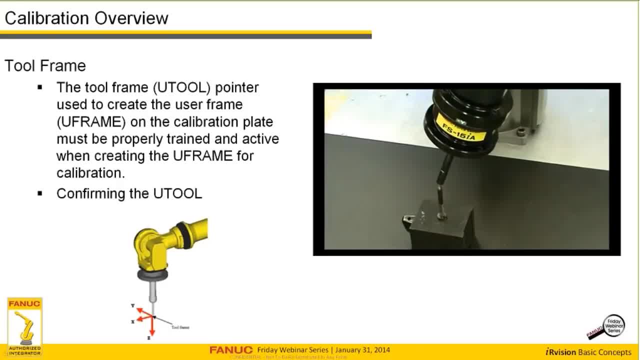 and then jogging the robot in yaw pitch and, as we will see here in a moment in roll, and verifying that that pointer maintains its absolutely correct relationship to the tip of the object that we're pointing to. This confirms that we have a correct pointer. 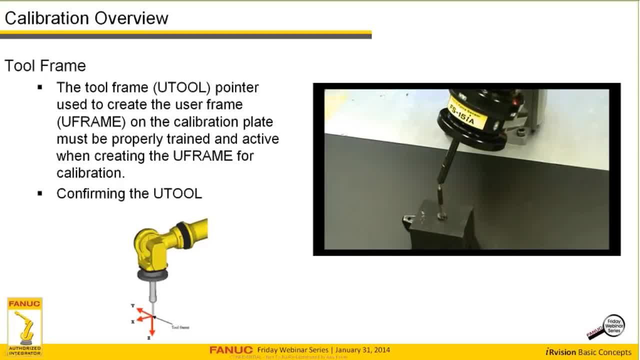 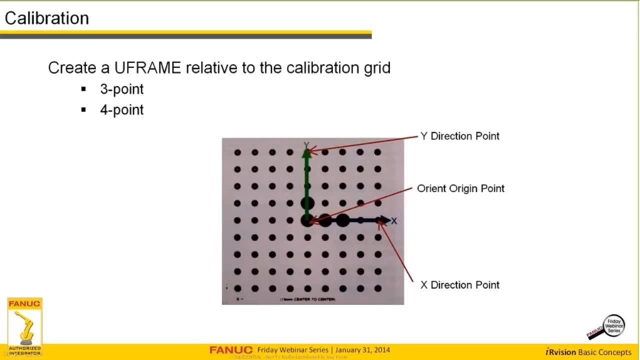 and one of the ways you can really mess up a calibration is to have an incorrect or incorrectly specified pointer when we're touching up the U-frame for calibration grid, When we create a U-frame for a calibration grid, we have to work with the actual calibration grid as touch-up points. 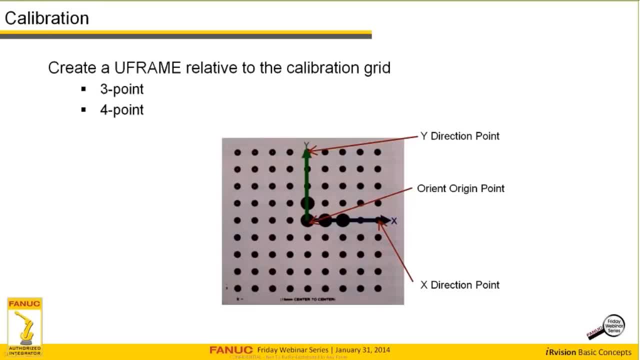 As you may know already, there's a three-point and a four-point. There's a three-point and a four-point. There's a three-point and a four-point. There's four-point. training for a U-frame. training method for a U-frame. 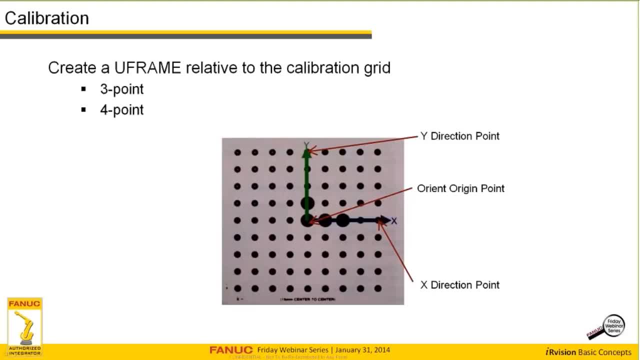 and there are specific points that must be used on the calibration grid for each of these training processes. If we work with a three-point train, the Orient origin point will be at the center of the large dots in the calibration grid. The Y-direction point will be the furthest most Y-point. 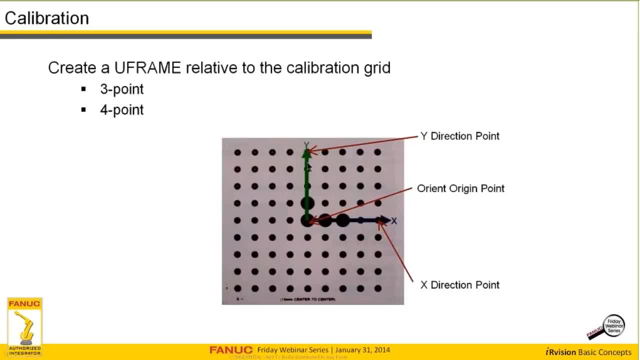 specified by the two dots, the two large dots in the middle of the grid. in the positive Y direction, the X or direction point in the u-frame training will be the furthest most X point, as signified by the positive X direction indicated by the three main big dots in the calibration grid as well for a four. 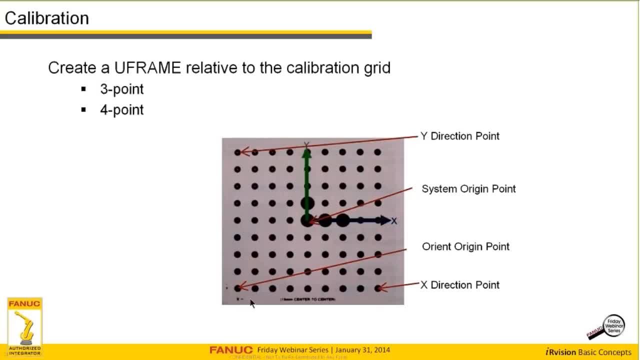 point train. it changes slightly. we use the least most point on the calibration grid relative to those to that L. for the orange origin point, the furthest most X direction point along that line of dots. for the X direction point, the furthest most Y in the same, in the same manner for the Y direction and the. 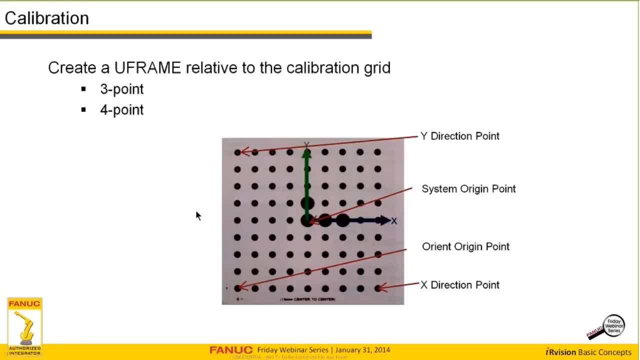 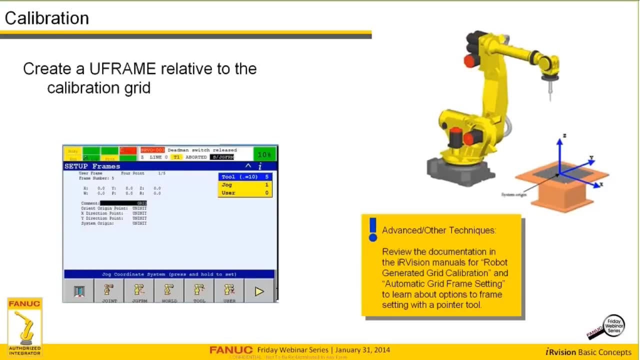 centermost dot becomes the system origin point. so let's look at how we will approach an actual calibration using a grid frame. calibrate a calibration grid frame. first thing we do is go through the teach pendant to set up frames and select the user frame that we're going to, that we desire to. 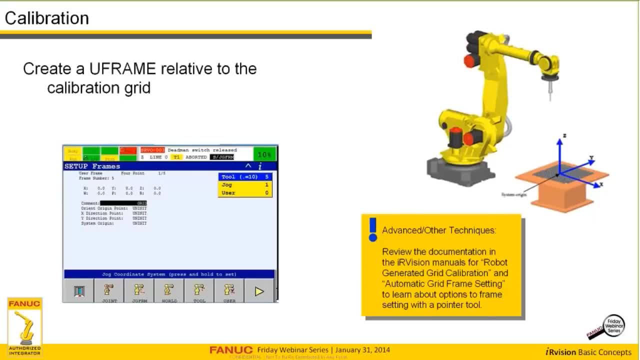 train as the grid calibration frame. in this case, I've selected user frame five and we want to make sure that that tool that we just confirmed earlier is the tool that selected that we'll be working with as we train the grid frame points. we will make a comment here. I called this the grid frame, the. 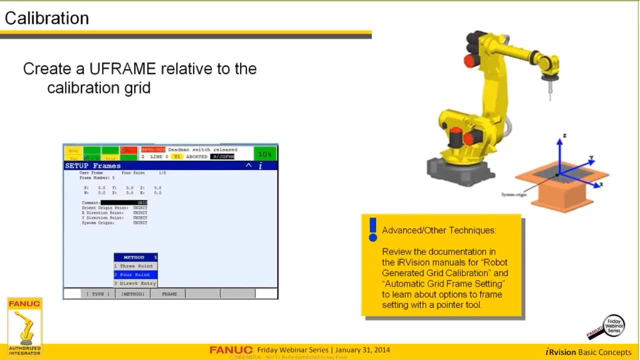 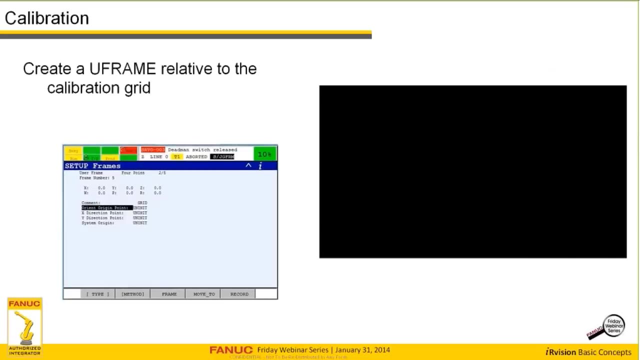 grid user frame and again verify, even though it's already up at four. four points T method. verify that we're doing a four point user frame. teach from there. we position our cursor at the orient origin point and we'll start moving our robot. now we're going to jog the robot again. 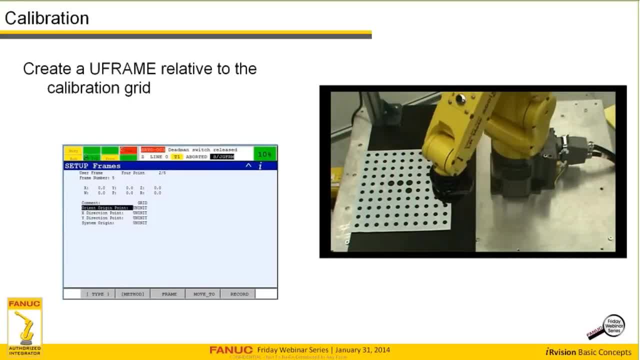 making sure that we've selected the tool that's been confirmed and the tool that we're, that it's related to the actual pointer that we're using and we'll move that pointer to the orient origin point, which is the least, most point relative to the positive X and Y direction of the calibration grid. well, carefully, I'm. 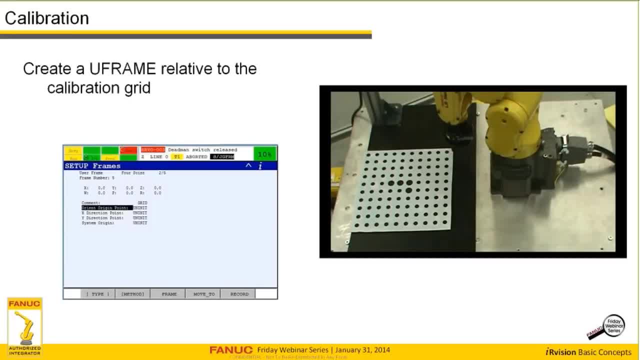 going to carefully move that pointer so that it's centered directly over the over the dot, also making sure that my X or in X direction is right at the surface of the calibration grid. when we have it in place, I'll press record and that point will be recorded and I'll move on to the X direction point now, jogging in world. 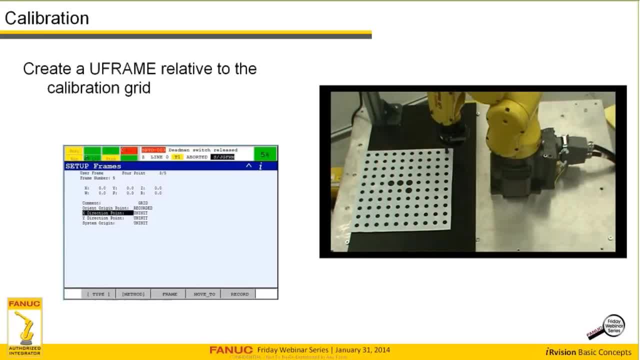 coordinate makes this a little easier. we'll move the robot to the X direction point, the furthest most X direction, in the positive direction, as indicated by those three dots in the middle of the grid, and once again carefully position that that pointer over the center of the dot. 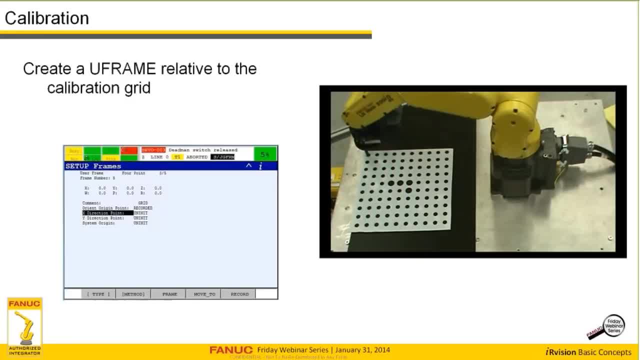 moving it in Z. so it's just touching the calibration play and once it's in place we'll press record and that will record the X direction point moving down to the Y direction. then we'll again jog the robot to the Y direction point, the furthest most Y direction relative to the orient. 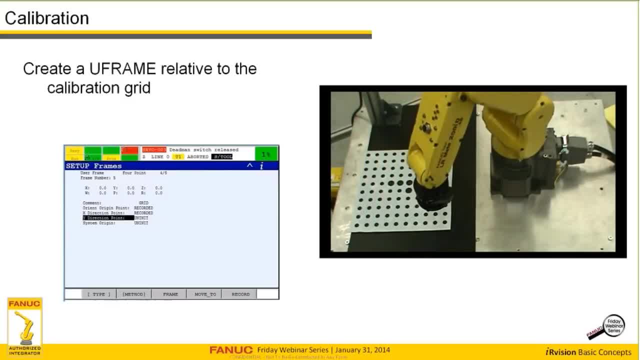 origin point and carefully move the pointer again to the center most point of that dot and record that position. finally, we'll repeat this same process with the center large dot on the grid which is the system in the four point peak. that's the system orient, system origin point. 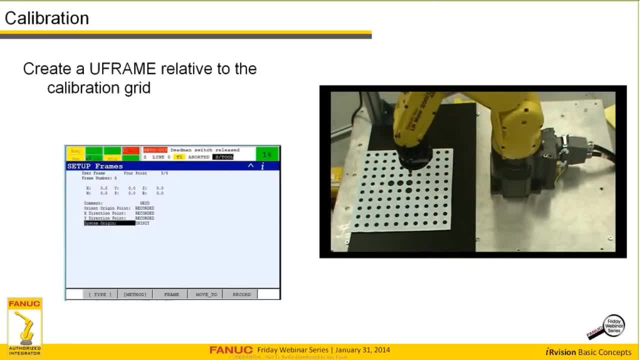 as we go through this process, I want to point out one more thing. the calibration grid must be at or near the z-axis height of the parts you intend to inspect. the surface of the parts that you intend to inspect, some error is allowed, but in the type of calibration we'll be doing, it's critical that you. 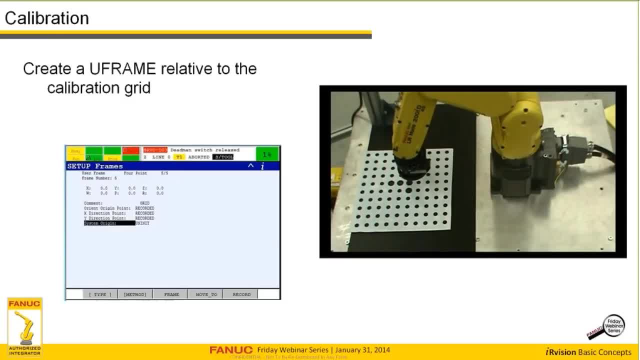 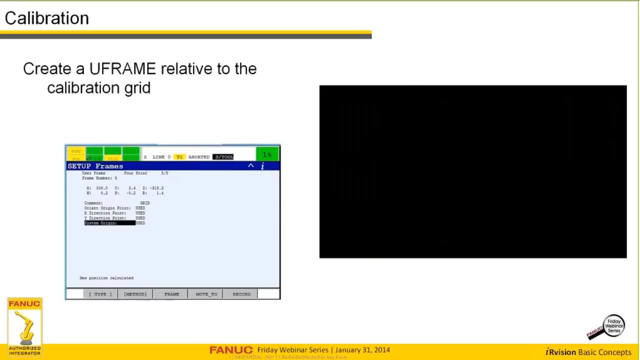 get as close as possible to the z-axis height of the target parts. once that system origin is correct, we'll record it and you see that the setup frame has been a new position has been calculated and all the points indicate that they are used for in used in that user frame. 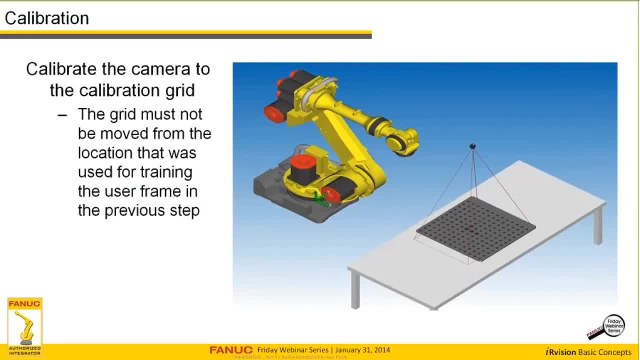 our next step is to calibrate the camera to the calibration grid and I'll make one critical point here: that you have to put a big circle around and make a big model in this type of process. the grid must not be moved from the location you that we use for the 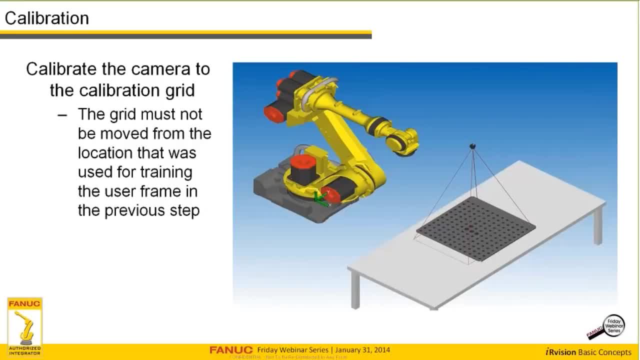 training in that previous step. I find it useful in an application and on the plant floor to actually pin and position that calibration grid in a way that you can remove it and replace it so that it's accurately are accurately manipulated in the case that the camera needs to be recalibrated. that can save. 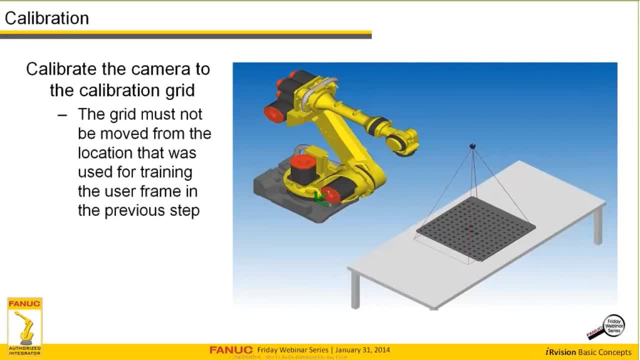 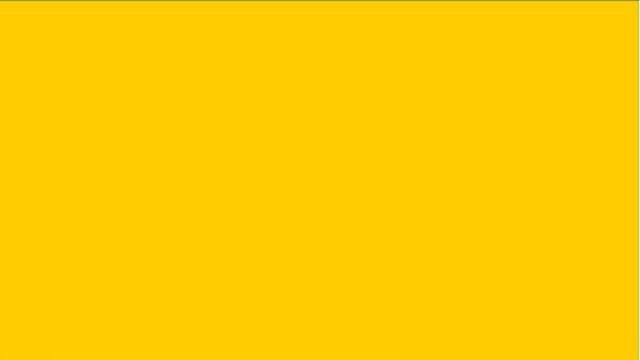 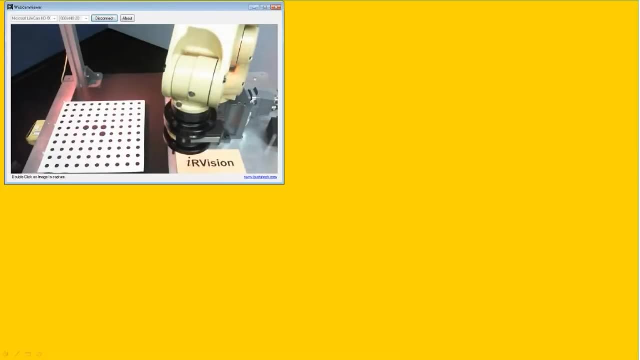 you from going through the manual grid frame calibration and touch up should something happen to the camera or the system. so what we're going to do now is go to our live setup and you can see our robot through our webcam, our IR vision webcam on the upper right hand side of the 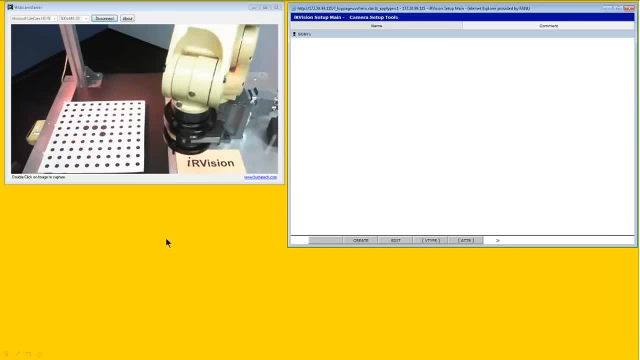 screen and I'm going to bring up our IR vision setup environment now. for those who are not familiar with this. the IR vision setup can be accessed from the FANUC robot web server or from: if you're using the R30ID controller, you can also do this process. 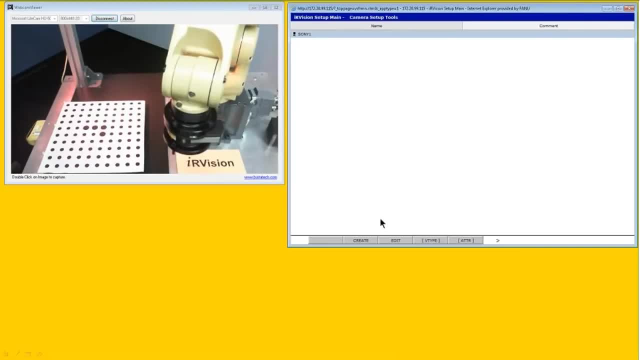 right on the teach pendant. this is the newest IR vision setup and if you have an older version of IR vision things will look a little different, but the overall theory will be the same. in operation we, as we go into the IR vision setup, we see that we have a one camera setup tool already present. 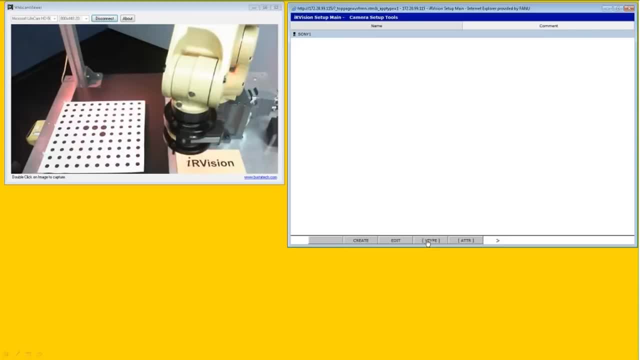 we'll set up this camera and hardware, and we won't go into how we actually have to do that. that's an easy process. you can look at the documentation. what we want to do, though, here is select from V type a camera, calibrate the camera calibration tools, and we'll create our own camera calibration tool selecting. 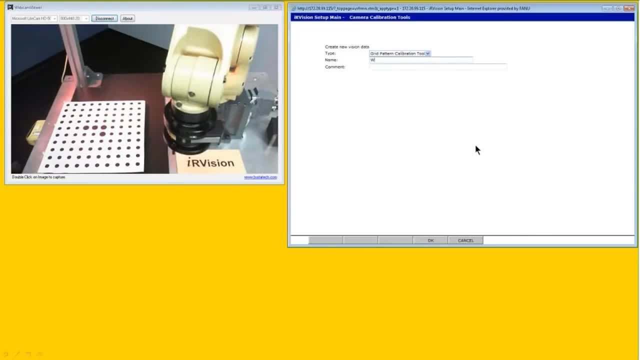 the grid pattern calibration. we'll name it something useful and even give it a hand. and with that we've created a camera calibration tool. let's edit that camera calibration tool and walk through how we will do our camera calibration again. what are we doing here? we're relating the camera field of view to 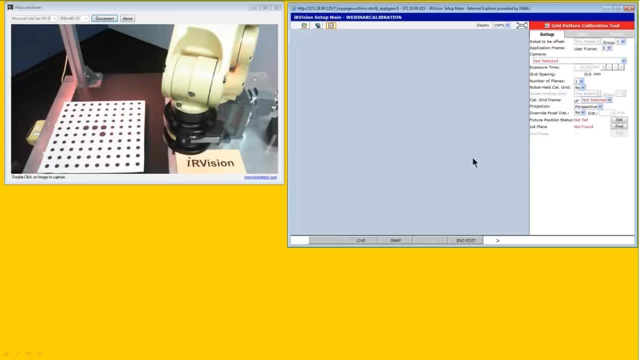 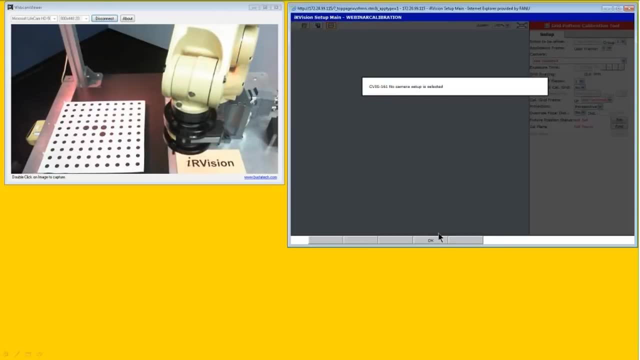 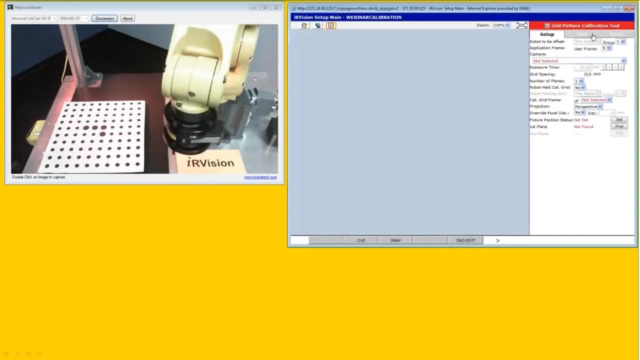 that grid that has just been trained. the robot knows where all the points are. we now want to tell the camera to know where the points are in its space. a snap a picture. look inside. we're going to have to be. we snap a picture. we want to do a couple of setup processes here, first of all. 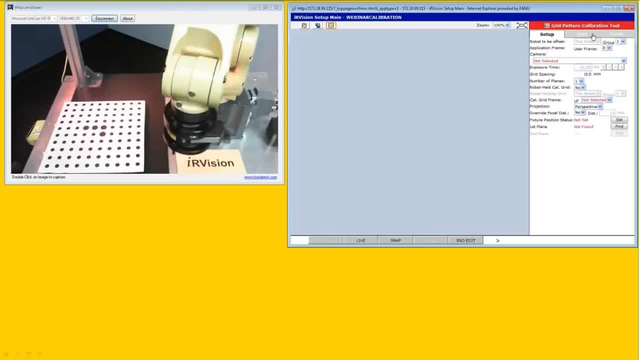 we're going to select the application frame. I'm going to use application frame five. that's arbitrary, that you can use a different application frame, but once you've set it in your calibration, you must use that application frame in your pic process. I'm going to select the camera that we previously set up, which. 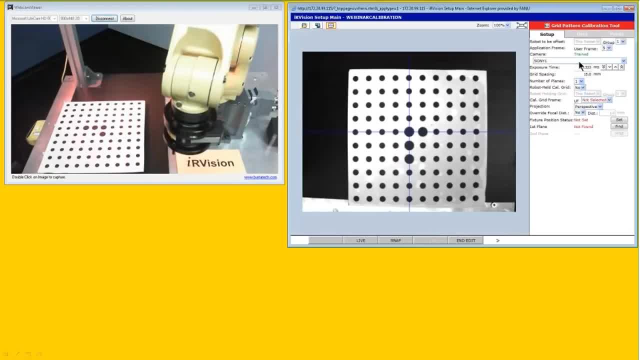 is the Sony one camera and make sure that our exposure time is adequate to see this. see this calibration grid. well, our default of thirty three point three, three, three milliseconds looks correct for this image. we also it's critical to set the grid spacing for the grid. we know, I happen to know, that this grid is. 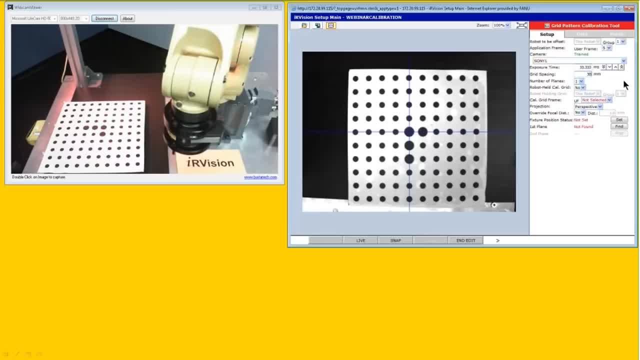 30 millimeters. your grid will be different and it typically will be listed on the grid what the dot grid spacing is for your spacing and the dot grid spacing is for your spacing specific grid. a few other count, a few other parameters to be used. we are only 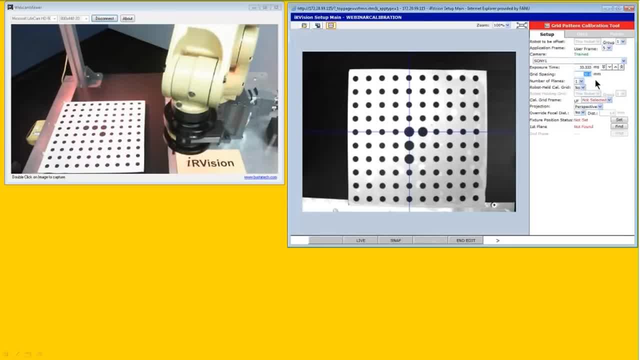 going to use a single plane calibration again I. some of the other types of calibration are for more advanced topics. the calibrate calibration grid in our case is fixed to the table, not robot held, and the grid frame. again, the frame that we just taught through our touch-up process is user frame five for our 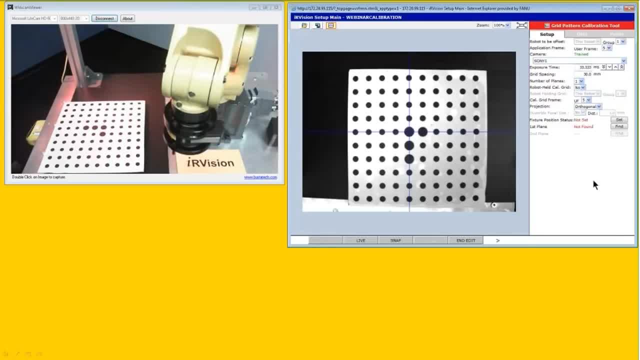 beginning, introduction, introduction to This: 교 gauge is advanced with a new set of bidi we are teaching, which is the request program for Earth and the, which would be the next-generation instrumentation which by not oh, oh is our, is to be the ribbon, error based and. 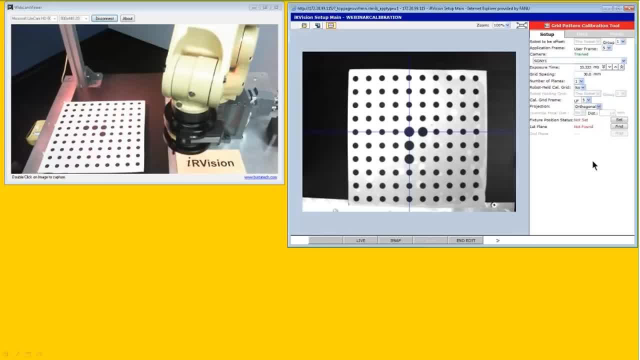 we're gonna be putting in those, this, the area definition, which, exactly after the correct for some of those errors in the calibration process. first thing we do, then- and it's very simple to proceed- we're going to set the fixture position status. what this does is, through a single click, relates the user frame that 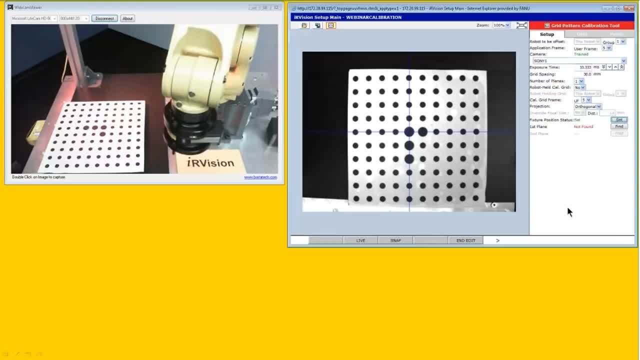 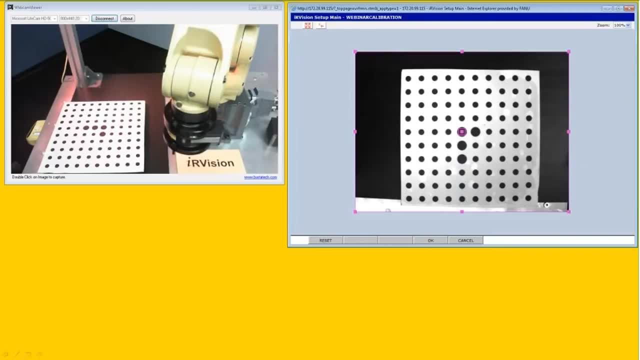 we've selected user frame 5 with this camera frame, and then the only thing we need to do next is to train the dots that are found on the grid. so we select the find button and this is a region of interest. I'm going to manually drag this. 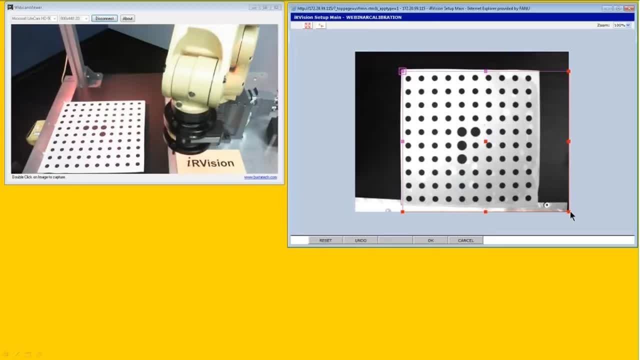 or position this over the calibration grid so that the region of interest is just outside of all the dots, yet not touching any extraneous black features that could confuse the find process. I'll click OK and from there the process will automatically find all of the dots on. 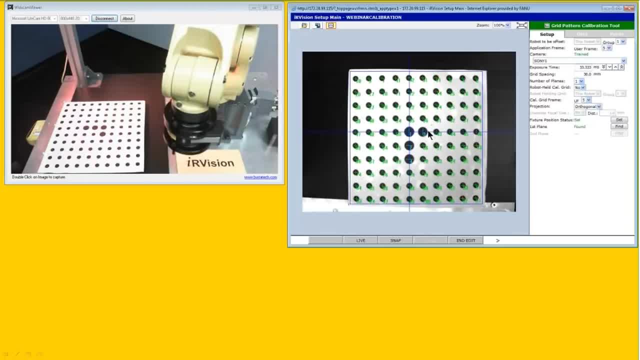 the grid and correctly order them in reference to the positive X and positive Y axis. we can check this out by looking at the data tab and we can see that the one, one value in particular that I like to look at is the mean error value indicating a point one, three, eight mean. 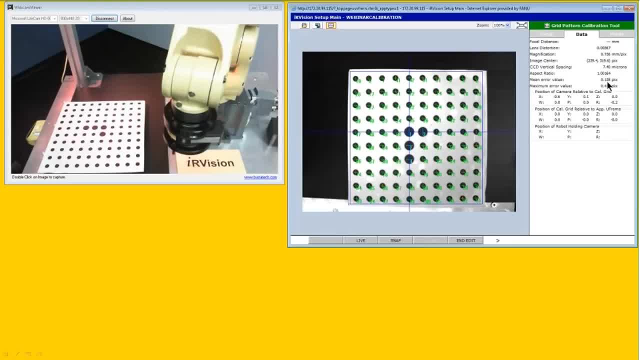 error, which is a very good calibration. anything below 0.5 for most applications is pretty good and for some applications evil, even over a pixel, can be acceptable. we also can look at the points. I want to show you this because it relates well to that table I showed you earlier where we have a vision, vertical a vision. 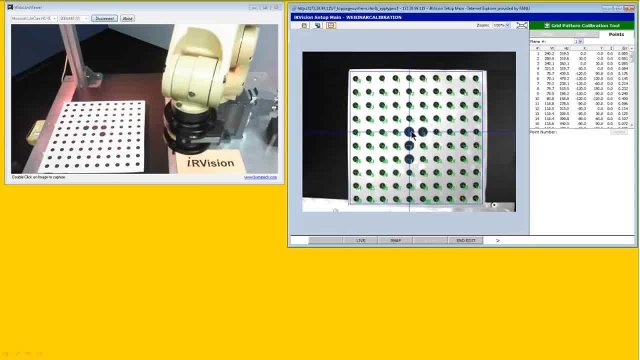 horizontal position and then the real-world position of these points, just as we would expect from our grid frame train. from there, we only need to save and I always remember. I always try to remind everyone to remember to save your tools and your processes as you go through them. that's one of the biggest. 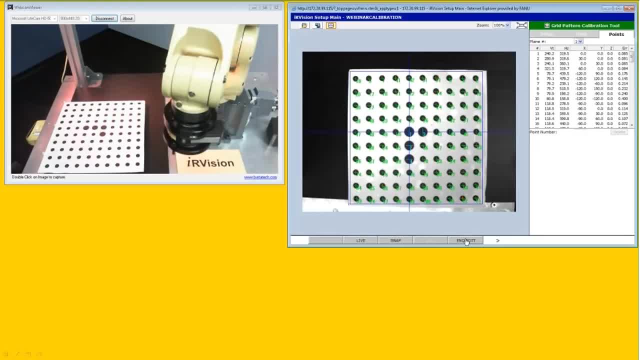 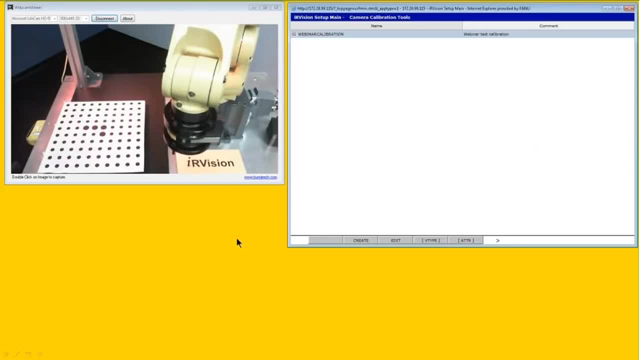 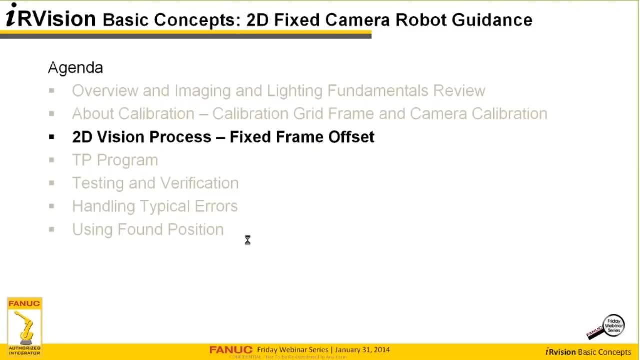 mistakes I've seen have being made and we'll end the edit there and now we have a successfully calibrated robot system. you I'm going to show you how to calibrate a camera with a correctly trained user for a user frame and a correctly calibrated camera. where do we go from here to finish up our process? and you're going to not. 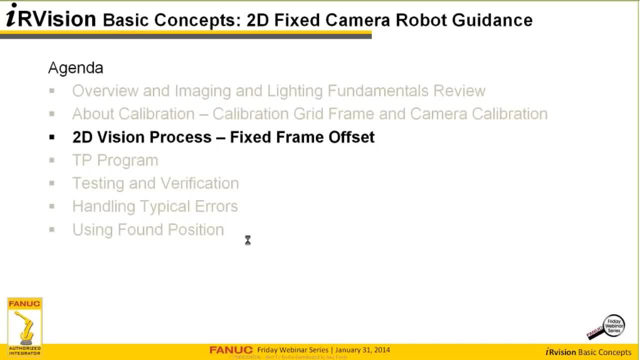 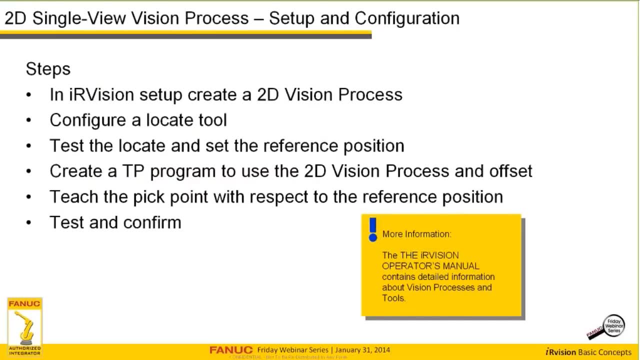 believe how easy this is. we're going to talk about now a 2d fixed fixed camera and single view vision process using fixed frame offset steps in going forward in this process. in our vision setup will configure a locate tool, test that location and then set a reference. 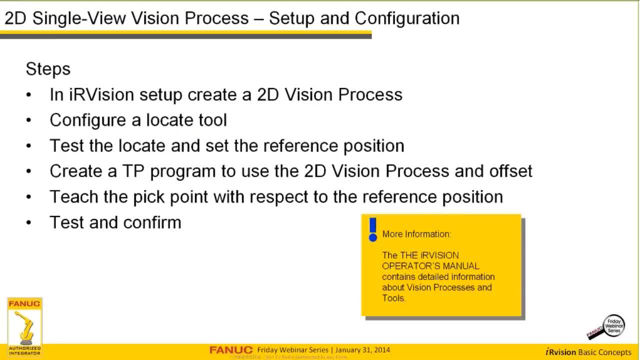 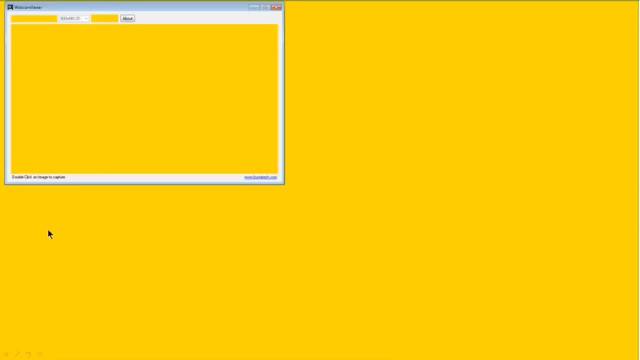 position- and very important and we'll talk about that in a bit- and then we'll create a TP program to use that process in that offset, teaching the pick point with respect to the reference position and then test and confirm our overall tick process. that's once again bring up our live web browsing. you can see what we're doing. 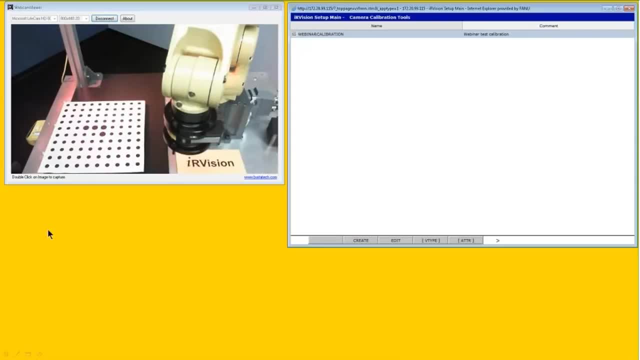 will look at our IR vision setup and I'm going to remove, now that we're done with this, the calibration grid, showing you one important thing: that the calibration grid is indeed set at approximately the height of the part that I'm going to be working with. I used a block to make sure that that calibration grid was at the 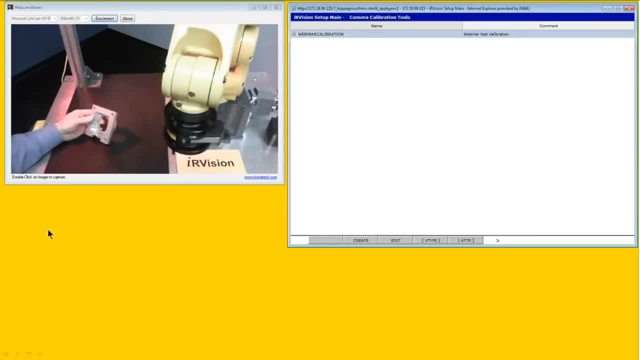 right height and the part we're going to be located today is a simple machine part, pretty common, something that you actually might pick with the LRM8. it's a square about a square machine part and it has a channel here. the reason we wanted that was because it gives us an opportunity to look at 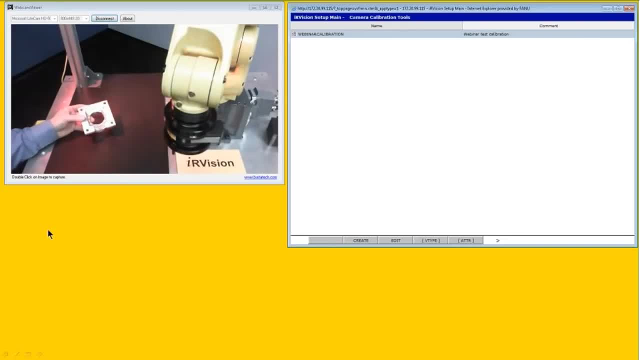 rotation. so we want to show that the system is going to do not only XY coordinate finds but also rotational forms. to get started, we're going to move our go in our IR vision setup to vision process tools and create a new 2d single view vision process. let's call that webinar to 2d. 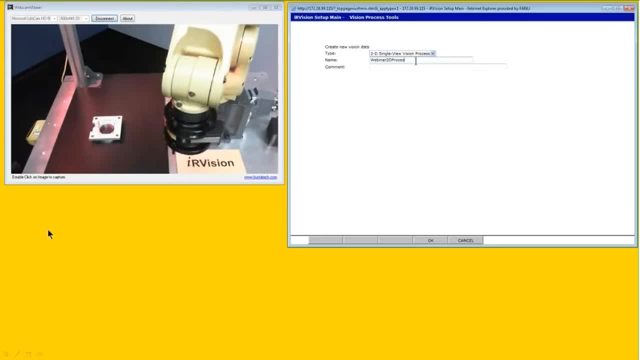 a process and we can give it a comment, and now it's created the process and we'll edit that process. starting out with the 2d single view process- again the familiar IR vision setup screen, we first have to select the camera calibration that we just work with and that calibration automatically brings in Sony camera. that 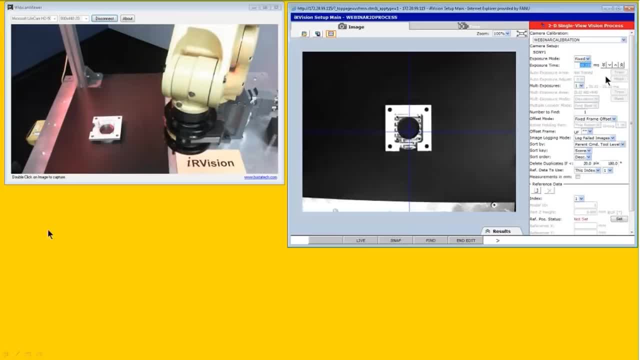 we configure, we'll take a quick opportunity to change our exposure time to optimize this process. for the part we have in place here, I'm going to make it just a little bit dimmer, but maybe not that dim, and of course this is some. the exposure time is going to be relative to the type of lighting that you're using. a 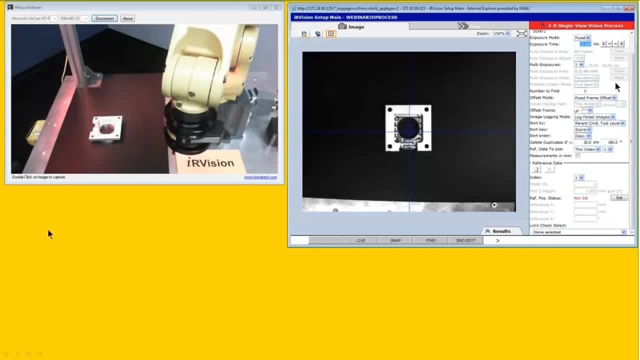 to configure, to finish configuring that single view vision process. there are a variety of parameters down here. I'm just going to point out the ones appropriate, important to our beginning process were first, to make sure we select the fixed frame, offset and again specify the offset frame, that frame number five, that 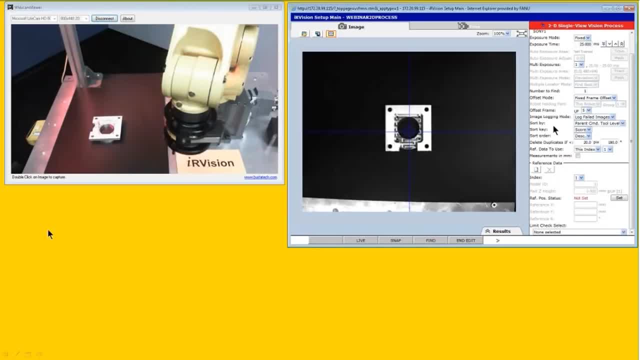 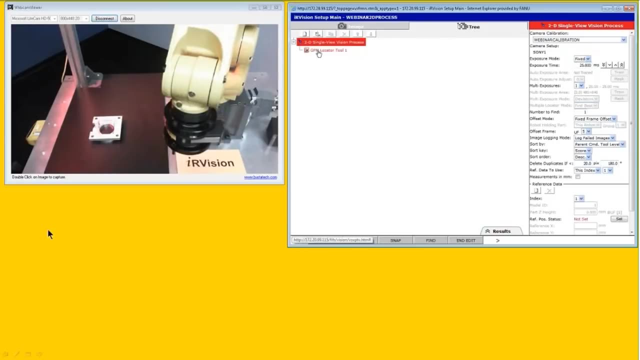 we trained earlier. that is going to be the frame that we put our read, that the vision process puts the results in and, And at that point we have the vision process pre-trained and ready to look at the locator tool. Now the 2D single view vision process automatically provides you a geometric pattern match as 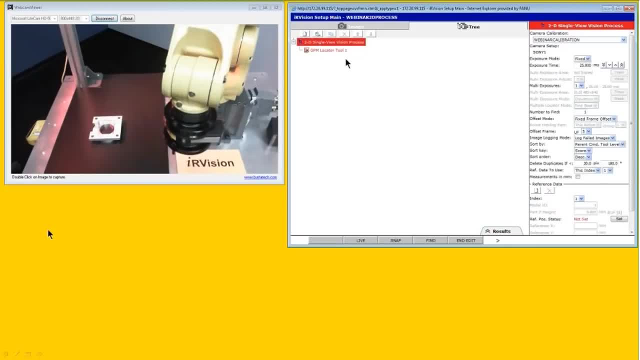 a locator tool, And that's a good locator tool to start with and may be appropriate for many of your easier 2D single view vision processes. I want to point out, however, that IR Vision is very flexible and has a wide variety of 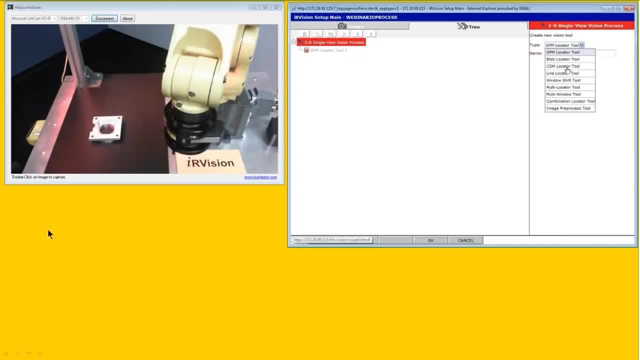 locator tools available: BLOB, CSM LINE and some other combination tools and more advanced tools that you can use to do more advanced applications and more complex location with the single view process. We'll address those, hopefully in another webinar in the future, but for now we're going to 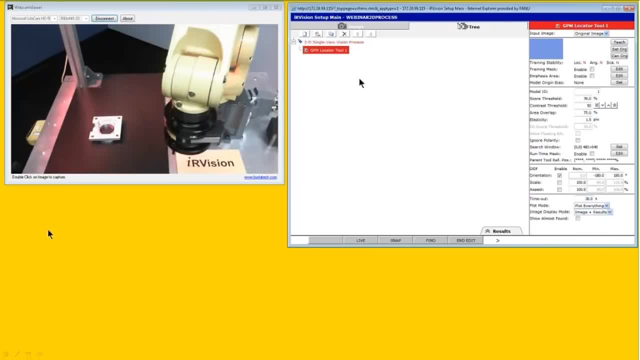 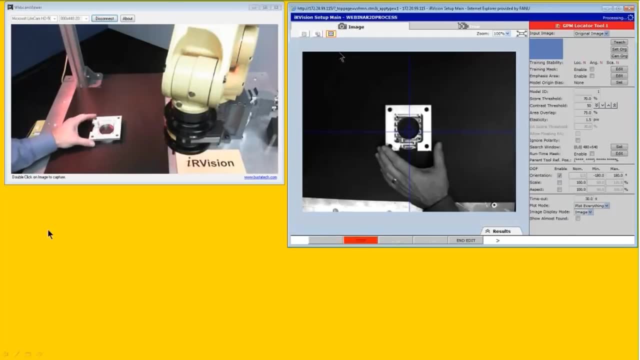 cancel that and stick with our geometric pattern match as our locator tool. Let's go to live. And I have our crosshair in the video, The crosshair that's available in IR Vision by clicking this upper button- And I just want to position that part in an optimal place. 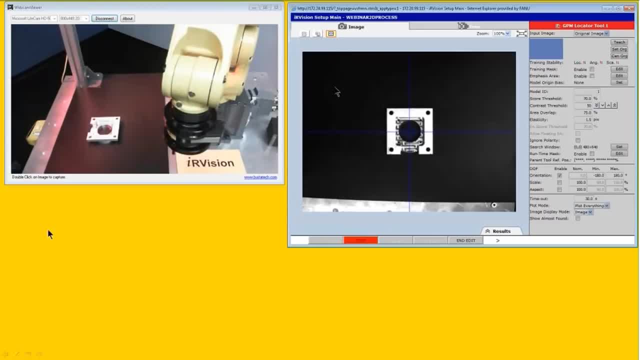 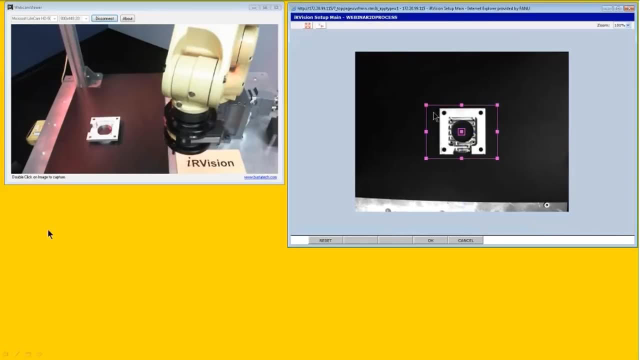 This isn't necessary, but if I have the part squared to the world, I find it makes it easier for me to train and understand where I've trained the part. The next step in a GPM locator is to teach the pattern. We'll go to the teach button in the upper right-hand corner, press that and it comes. 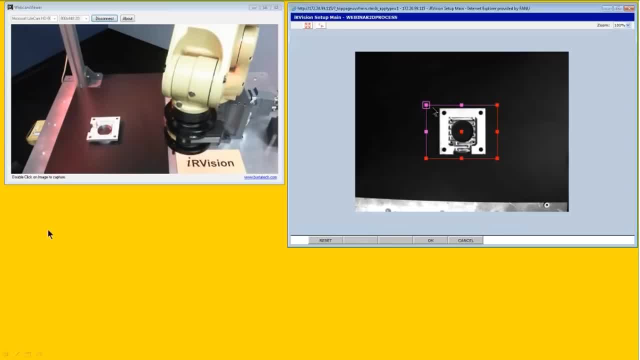 up with another region of interest that we can adjust And place. It says that we want to make sure that the color of our background is in the right place in our scene. I'm going to drag this section to the top. So I'm going to drag this section to the left. 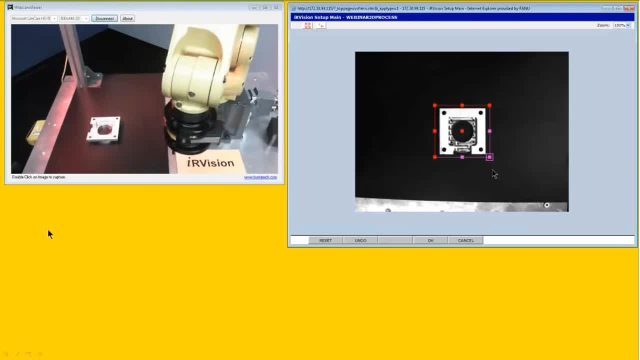 And right-click. I'm going to drag this section down And I'm going to select the end of the scene – this is the end and this is what we want to have in front of the scene, And I'm going to hold down the X key, click OK. 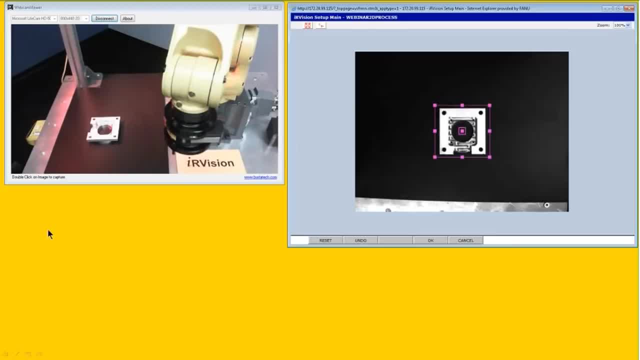 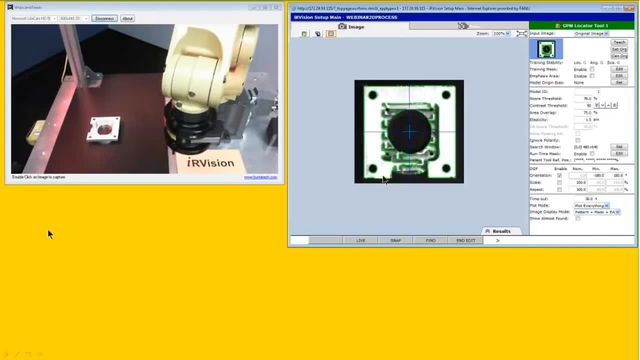 And then I'm going to select the view with the circles, And that's going to be it. I want to show you- And there we see- that the system has trained the critical edges of that part and placed the origin in the center of the training area. 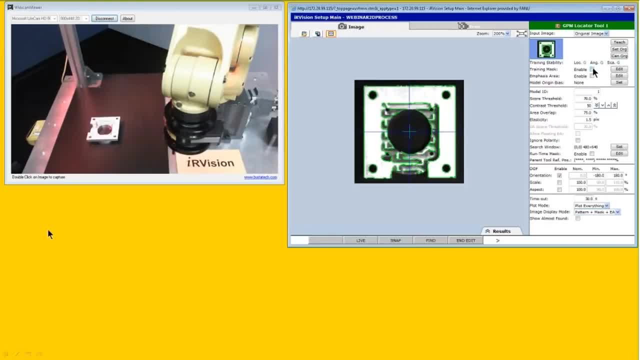 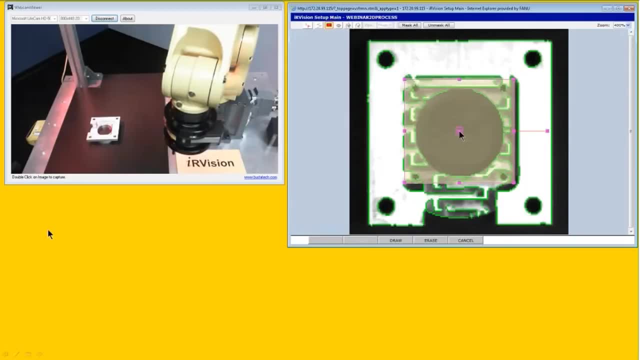 Now, since I'm not too happy with some of those edges, I'm going to set up a training mask to mask some of the unnecessary edges in the image, And we do that by placing a region of interest in the edit mask process around the edges that are not of interest. 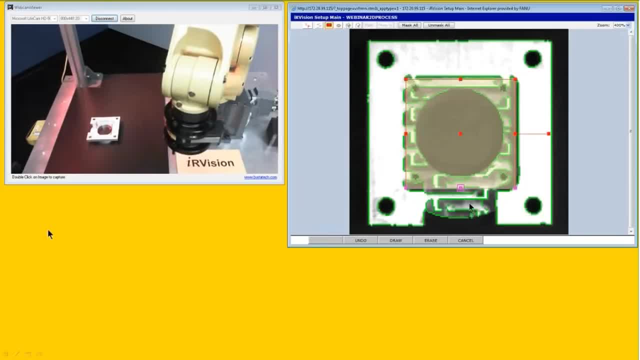 And why are they not interesting? Well, because they might not be consistent over a part-to-part basis. These are machining marks that are not going to be consistent part-to-part-to-part. We'll draw that in. And there's one other area I want to mask, and that's this opening. 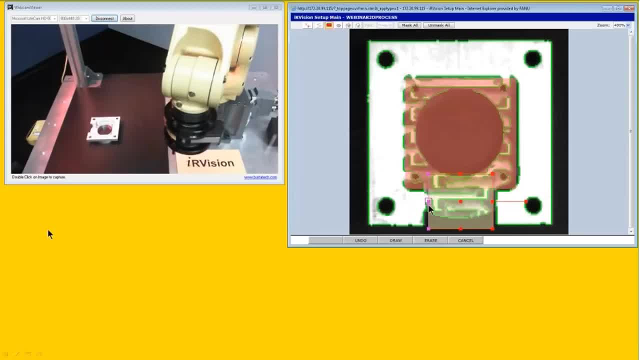 this cutout opening, Because that's going to be crucial. The accurate location of that's going to be crucial to finding rotation in this part. We'll draw that And with that masking we have a very well-trained geometric pattern. The one last thing we can do, if we wish, is set the origin. 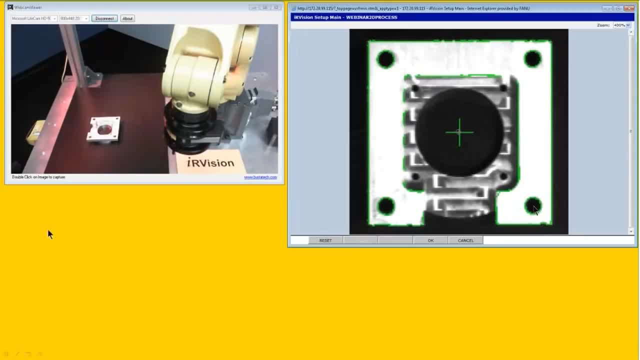 I'm going to have my pointer point to this hole. It's not necessary that I set that at the origin But again, to eliminate confusion, I'm going to point the origin And I'm going to set the origin to that hole and use that as my origin. 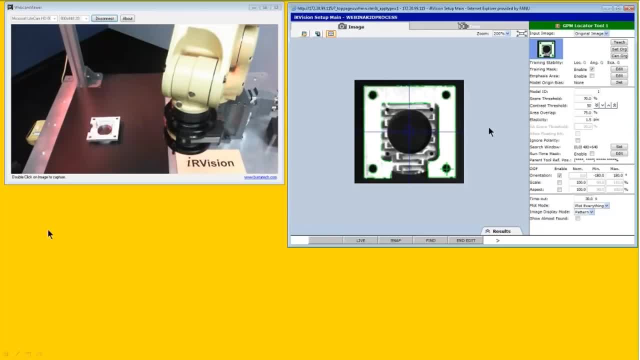 There are a lot of other parameters here. I'm going to leave that for another webinar and advise you to look at documentation to double-check that you know what to do with those parameters in a given situation. But for our purposes now we're going to do a snap and find and note. 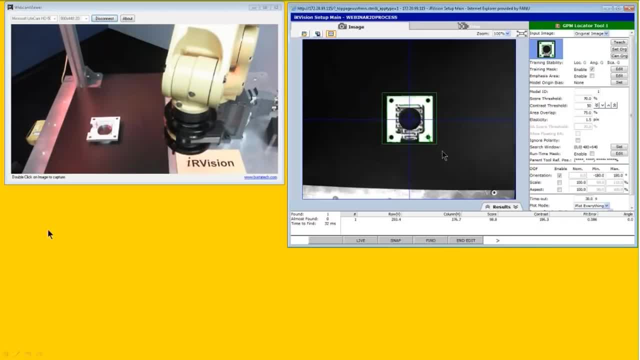 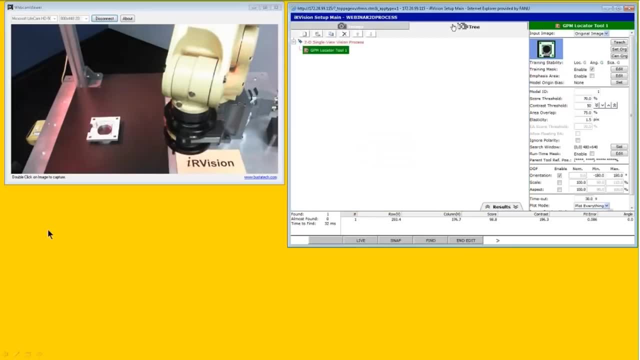 that the geometric pattern is being correctly accessed and very accurately found at 98.8%. Now that we have the pattern trained, let's go back to our single-view vision process. There's one more crucial step. Let's do a snap and a find. 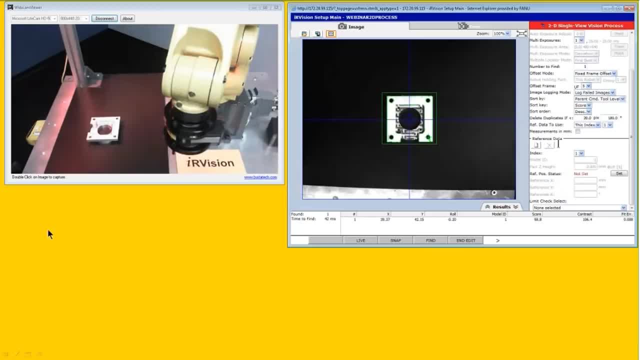 And the one thing we have to do is set our reference data. What is the reference data? The reference data in an offset, in a fixed-frame offset environment, is the point at which the fixed-frame offset will return a zero offset to our robot program. 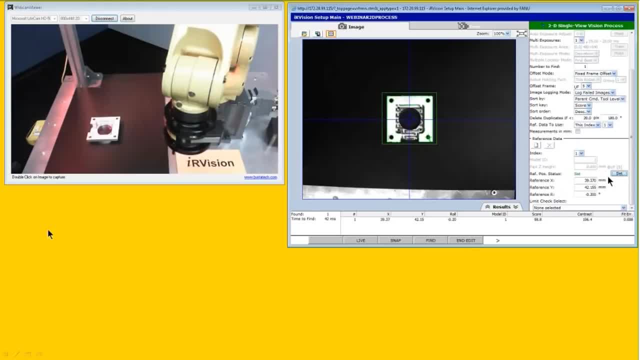 So when I set this reference data, this now, this origin point now becomes the point that is referenced at 0, 0. And we're going to use that to our advantage when we use the offset in our TeachPendant program. With that, our entire 2D single-view vision process is trained and ready to go. 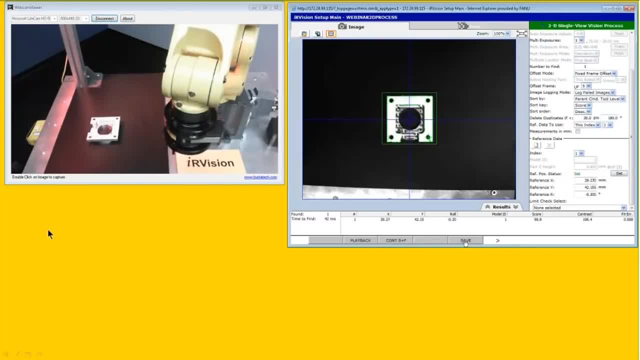 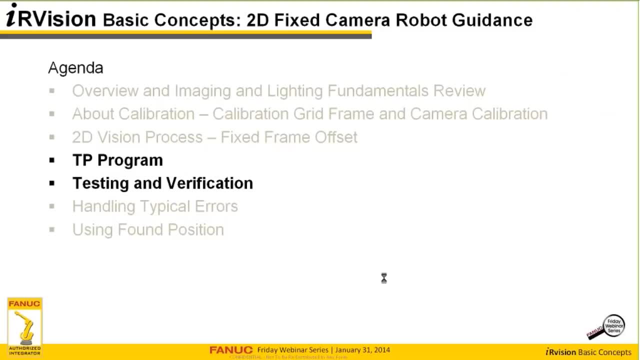 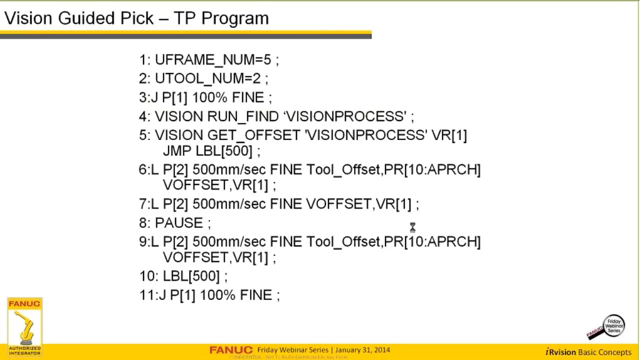 I want to remember to save it And we'll end the edit there and move on to the next step. Here we're going to be creating a TP program and testing and verifying the performance of our 2D vision process. Here's the PIC program, the TP program for a vision-guided PIC. 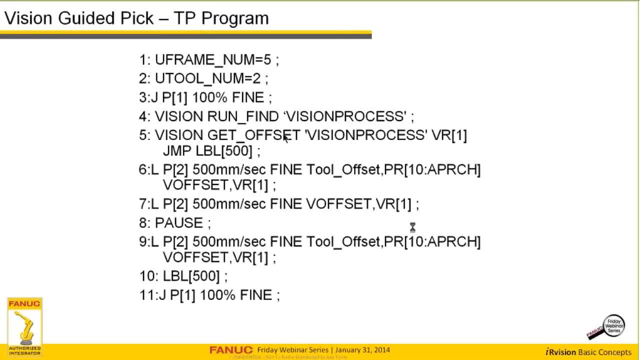 I have it already in place And I'll just want to go over it here. before we look at it live, We select our U-frame number. This is the same U-frame that I specified in my vision process And that is a critical number to use. 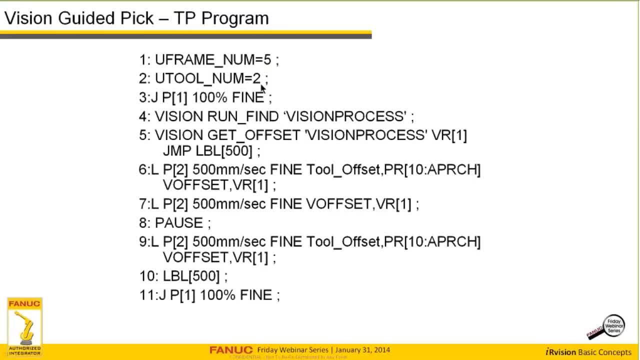 I specify a U-tool or a tool frame, And this number is not a U-tool. It's not so critical. All it requires is that the tool be a validly trained tool. It doesn't have to be the same pointer that we used in our grid calibration touch-up. 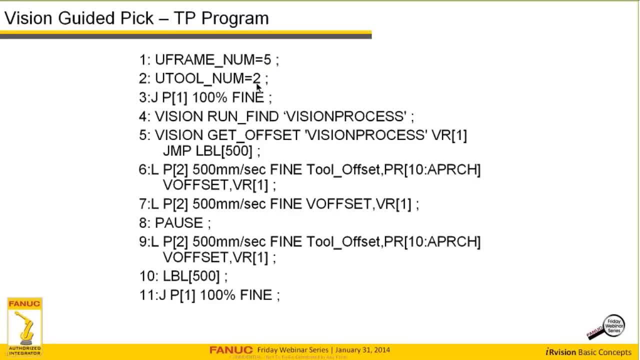 It just needs to be a validly trained tool. In this case, this happens to be the world tool. It's the faceplate of the sixth axis. I'll send the robot to a position that's out of the field of view. That makes sense. 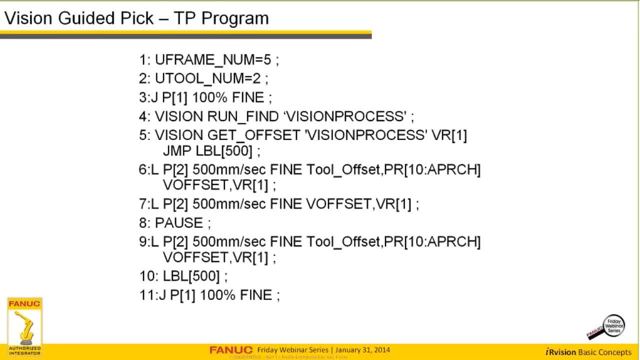 The robot can't be in front of the part when we take a picture And then do a vision process, which is called Vision Run, Find, And that is going to reference the vision process that we just created, our 2D vision process. 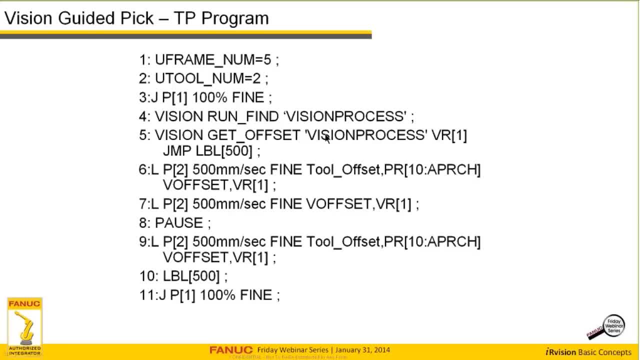 Then we'll do a Vision Get Offset which goes to that same vision process after it's found a part and pulls out the offset data relative to that reference position and puts it in vision register of our choice. If that fails, we want to jump to a label. 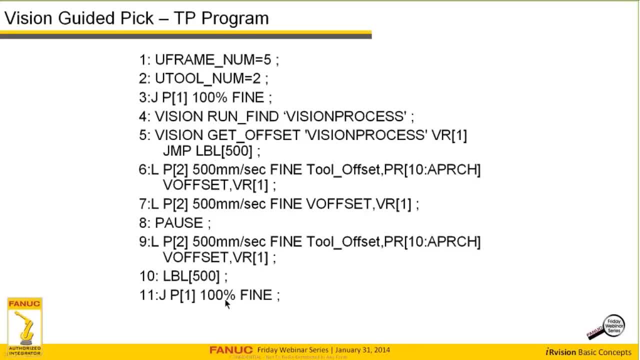 In our case, we're just going to jump and go back to the beginning. We then go to a trained tool. So I'm going to go back to the beginning here And we're just going to look up the level of the point, the point we just created here. 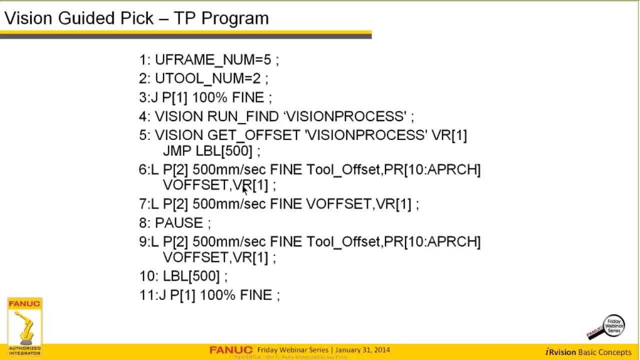 And then, when we're done, I'm going to click OK and I can go to the final tube. We can click the OK button to get to the final tool, the point we just created here, And finally, we can go on to see what happens. 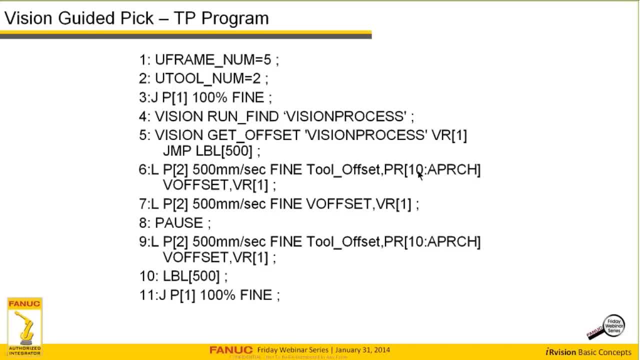 So now we're going to see the result. So we got the result being a 50 millimeter Z axis And we can click OK And we can do the same thing over here. We can hit OK And we can go back to the main node. 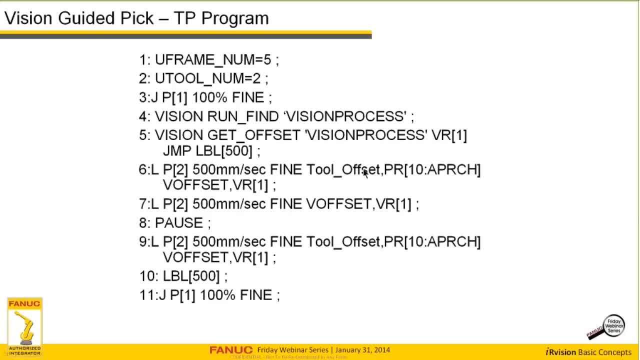 And that's all I'm going to do. next, We're going to check real-world. So I'm going to check real-world. So we've got much better and better results. I can see the results tool offset that has a 50 millimeter z-axis height difference. let's go to the 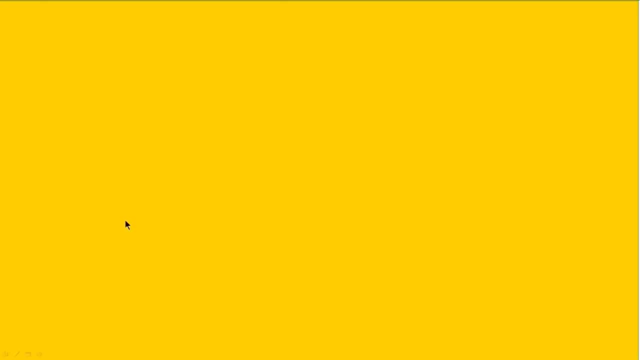 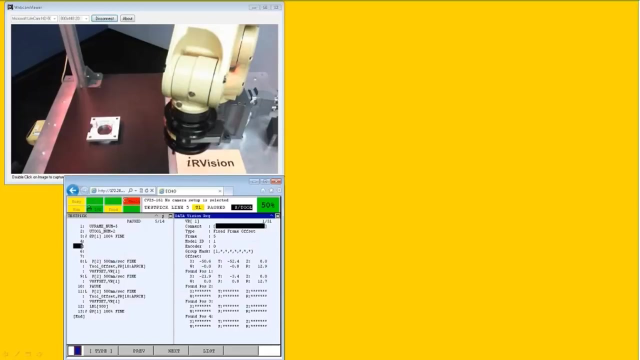 real world and see how this is going to work in the real world, let's bring up our webcam and our teach pendant and, since our vision process is already already trained, we'll just look at the runtime vision screen and see what we see, what the results are. so the first step you can see from my tool program: I 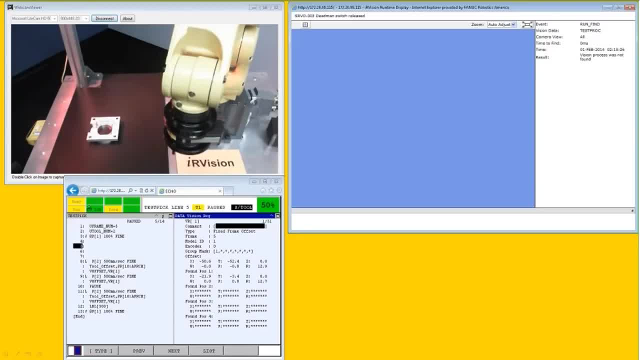 want to teach printed program. I don't have my vision things in there yet and I want it to show you how to edit the outer, insert the vision command, and so I'll pick the appropriate line and go to vision and the first, the first process is run. fine, I'll select choice and select the process that we just trained. 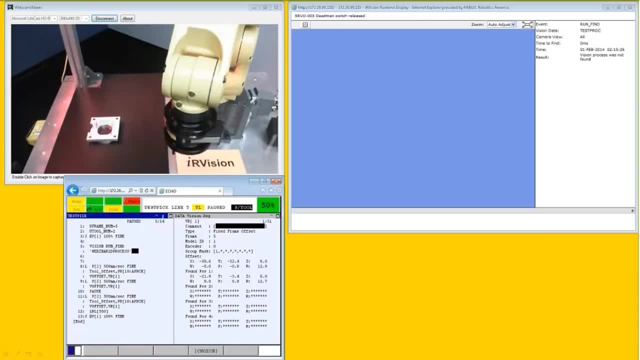 webinar 2d process. that, to find, is complete. now let's add in the offset gather. once again, going to the vision process and get offset. I want to select the 2d vision process that we just configured and we'll put this information in vision register one and, as we saw in the sample program, will jump to. 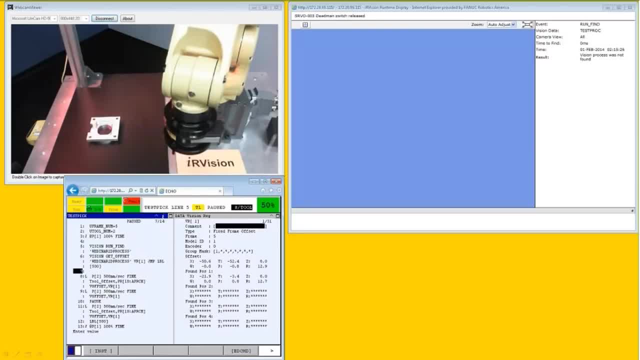 label 500. if that happens to fail- which we hope it doesn't- the first thing we're going to do is step through this program to perform the vision find and you'll see on the right-hand side of the peach pendant that I have the vision register data showing and what we want to see here is that the 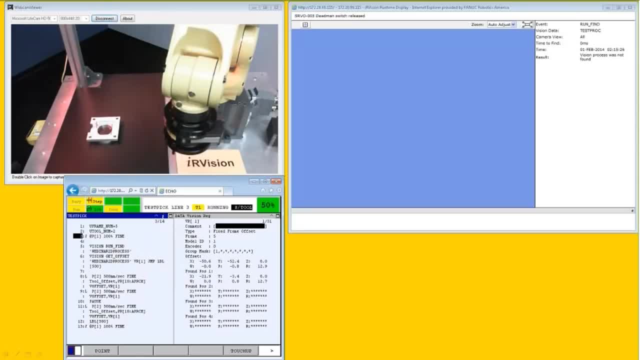 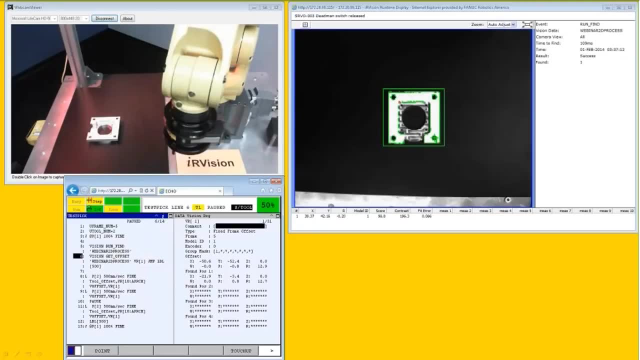 vision register when we get the offset, since we haven't moved the part at all. we haven't moved the part that vision register is going to report when we get the offset right here, it's going to report all zeros. that's an important step, noting that we have not moved the part, so it should be reporting all zeros. 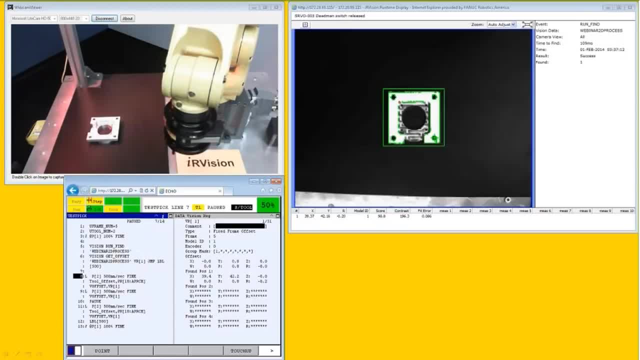 let's go down to our pick position and we will use, we will jog the robot to that pick position or to where we would like to pick the pick position to be, and touch that point up. oops, I'm going to use the touch up shift, touch up to touch P and that looks pretty. 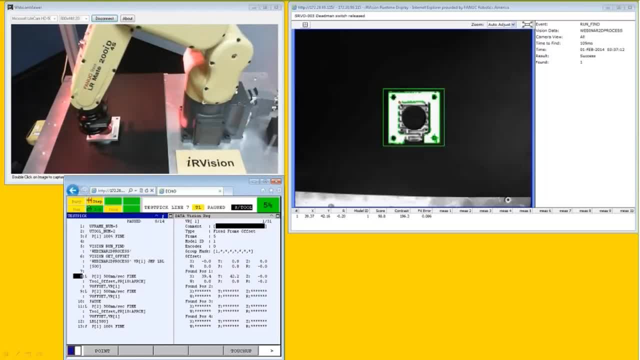 close. we'll call that good and I'm going to use the touch up shift touch up to touch P to such a P. to to the point I've just moved the robot to. we don't want to set a new ID and because we are at the zero position, I don't want to. I 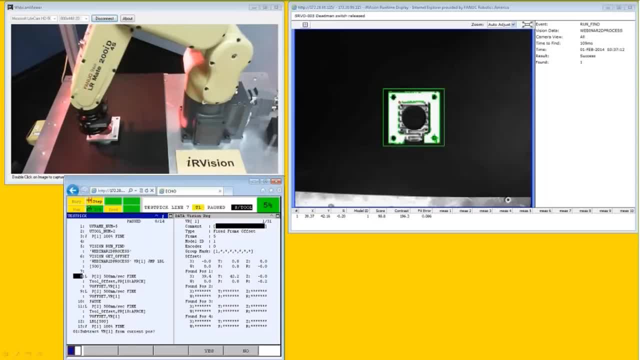 don't need to subtract the vision register from the position on touch up, and neither do we want to subtract the tool offset data from the position, from the position at touch up. so now we have a point trained. let's manually move away from that and I'll start the program over in step mode, just so we can see it run, the robot. 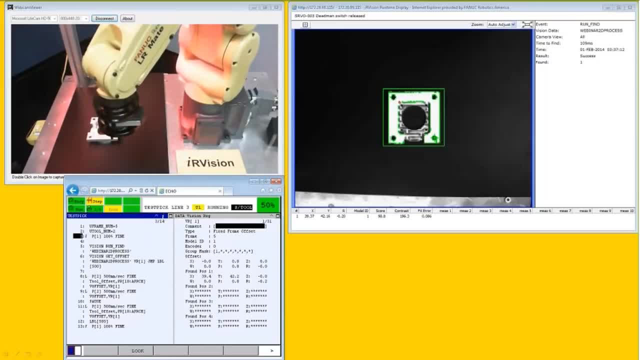 will first move out of the way and we're going to see over on the right hand screen of the vision runtime. we're going to see as we do a run find that data will update. it's not so easy to see because it's in the same place we'll get. 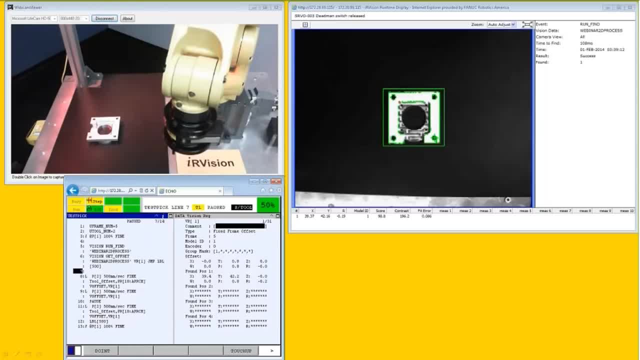 the prop of the offset, noting that it still is zero in the vision register. to the right, our pointer will move to an approach position and then down to find the part will depart and move back to the starting starting robot position, starting visit view position. let's try that now with just a simple offset in translation: 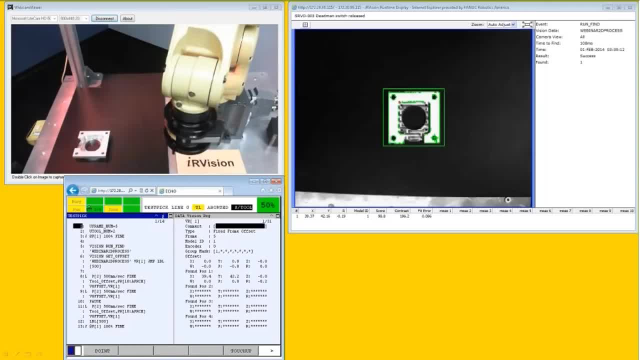 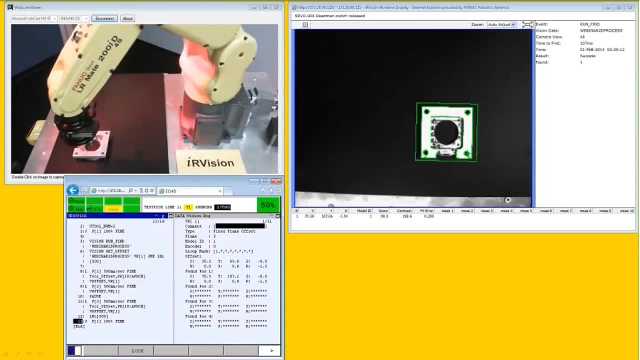 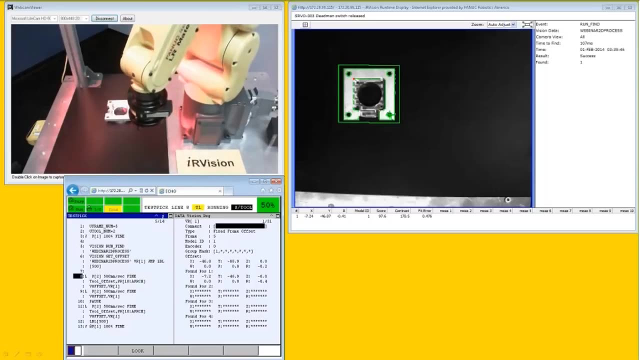 X and Y and we'll run the program in without step mode and we can see once again: perfect. that part has gone to the, to the position we trained, tried in another XY translation. that's great. here's the real test. let's add some rotation to the part and see. 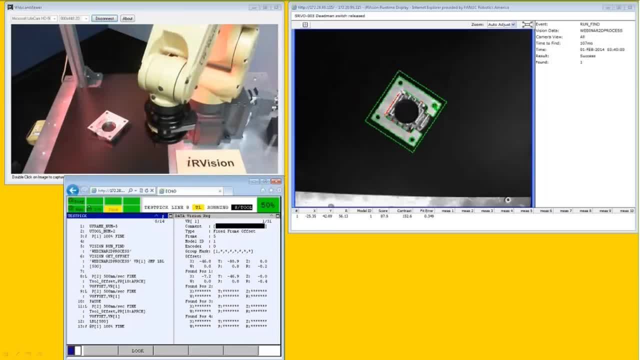 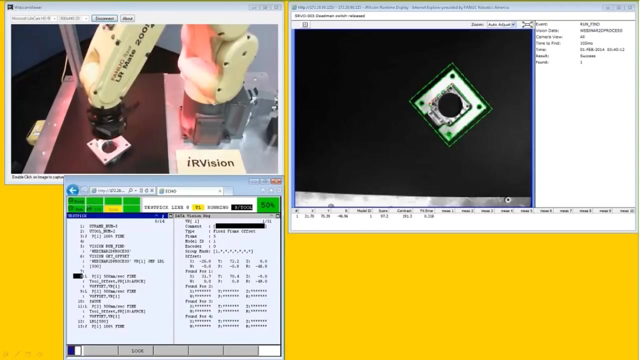 how the see, how the find works and, again, perfect. this is exactly what we want to see, as we, as we test, as we test and validate our process. we're looking at that. I have a question that just came in. the question is: when I go to a vision process, I'm not able to select the crosshairs or zoom in and out. 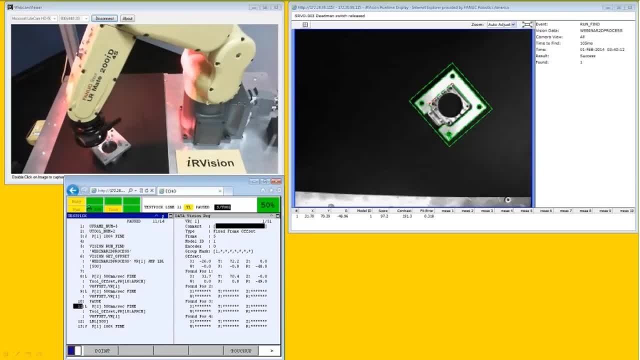 on the image. is there a certain version on IE that I need to be running to be able to see those buttons? I'll tell you what normally causes that. first of all, you do have to be running IE 9. 10 has not been validated and 11 has been tested, but IE 9 is the is the. 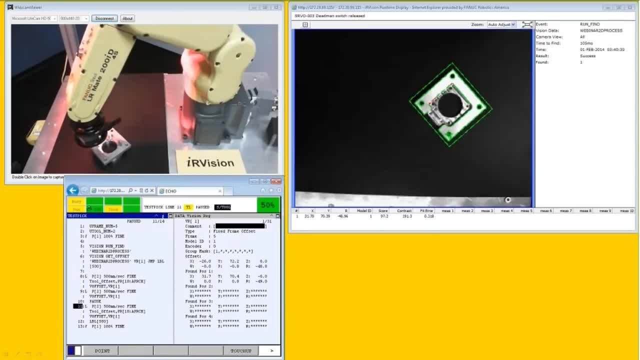 version that must be run. but there's another another thing going on there quite often, and that is you have to set your internet security options to to make the robot IP a trusted site. when the robot IP is not a trusted site may get some variation in the in the image on your vision setup screen. hey, let's. 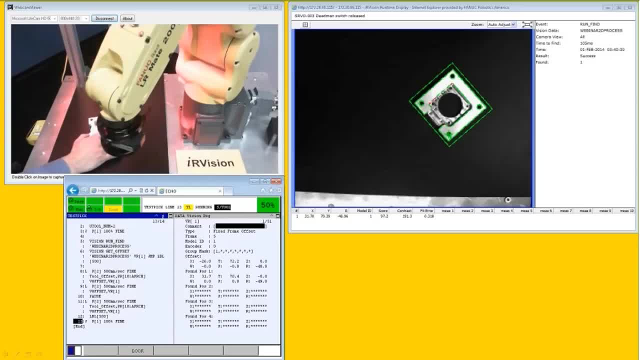 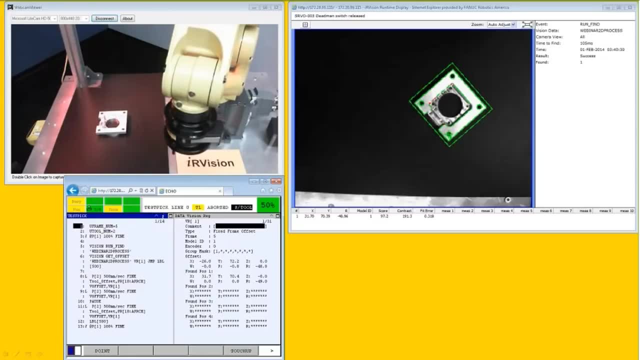 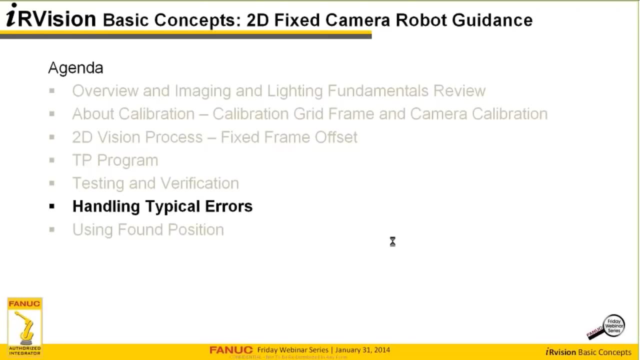 continue on great success there. we have very quickly created and found, created a vision process and very accurately found this part in space. so what happens when something goes wrong? I'm not going to spend a lot of time on this, but it's important to know where the errors can happen and where. 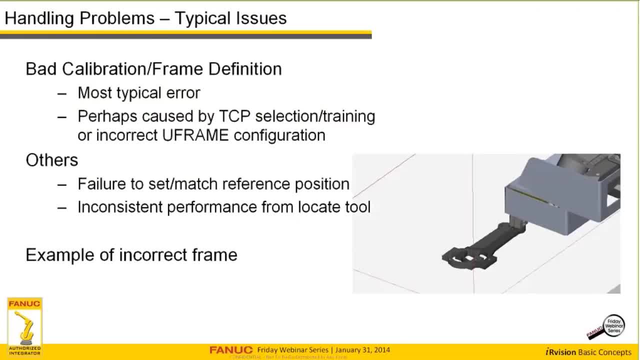 they occur. typical issues: most typical error condition is a bad calibration or bad frame definition. I would say that of the calls I get or the calls we get, this is the most typical error and it's usually caused by incorrect tool center point selection, incorrect tool center point training, and that what I mean by that is that you 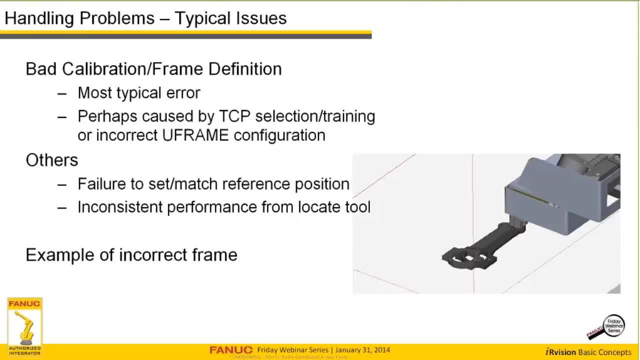 have not correctly trained the the tool center point and you have not, or you have not used the trained center point related to your pointer when you're doing the U frame configuration or incorrect you frame configuration are things like going to the wrong point, going to not matching the points to be to the desired space. so this is the 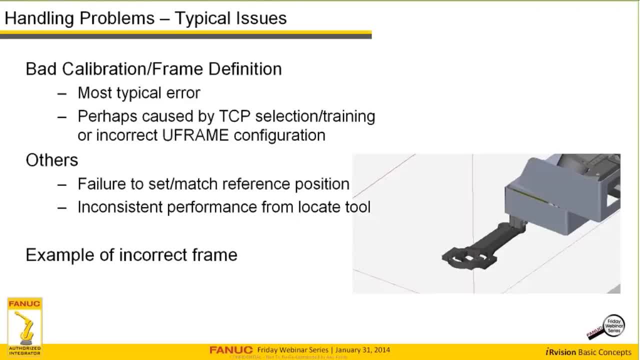 major reason we see handling problems. other possible reasons may be a failure. one big, big one is a failure to set or match up the record position. this happens quite often. that's in the vision process and, to a much, much lesser extent. inconsistent. performance from the locate tool that you've selected is a 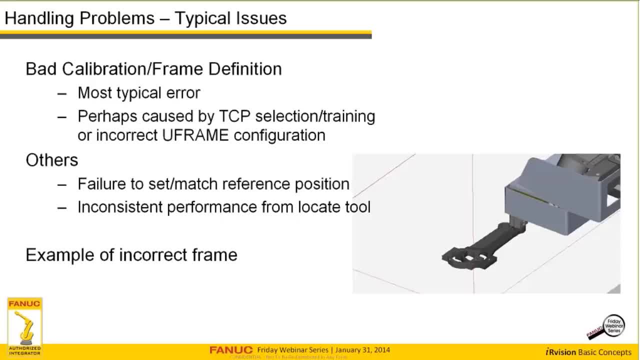 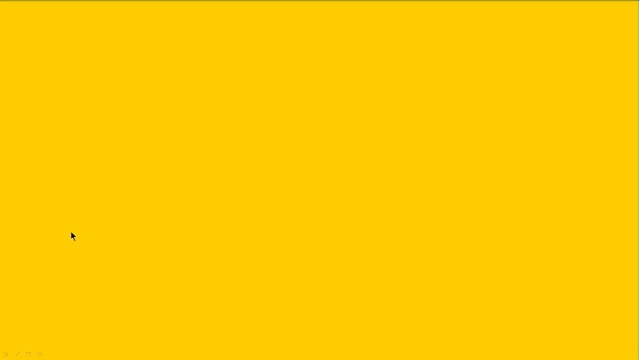 It's. this can happen, but if you do, if you do your testing correctly, you will likely Find that. Find that it's not a big problem. So let's both go and look at again in real world an example of what we might see when we have a problem. 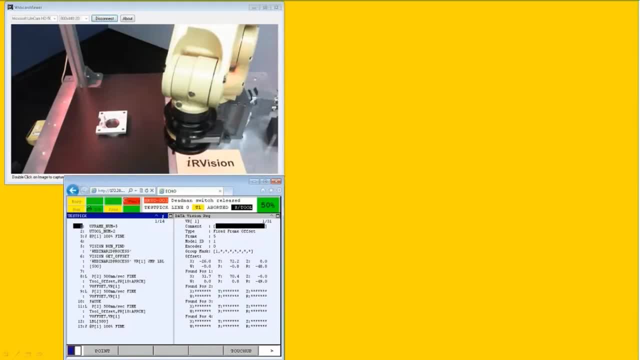 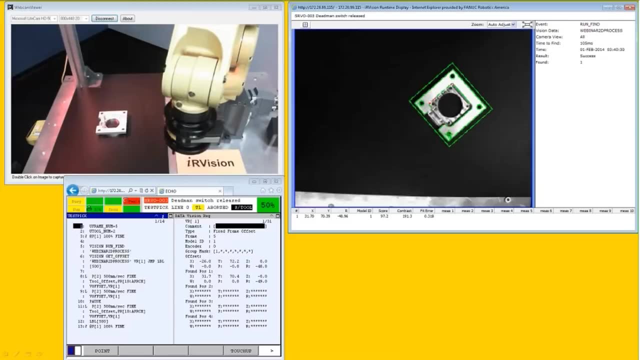 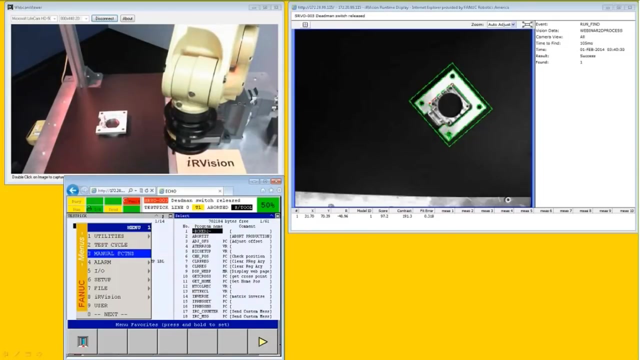 with With the frame or the tool point. I'm not going to take the time to actually Retrain my grid, but I'm going to simulate that. the way I'm going to simulate that is to go to the Grid frame that I taught And and in. 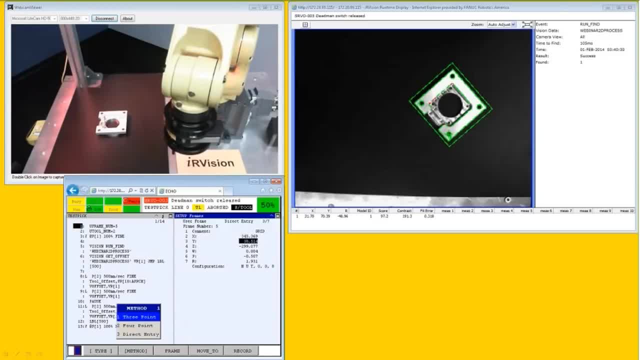 Under method and direct entry. Again, this is grid frame five. I'm going to change these numbers if you. I hope that you can imagine that You're going to. If I change the numbers on the grid frame, that kind of simulates the fact that you were possibly using the wrong. 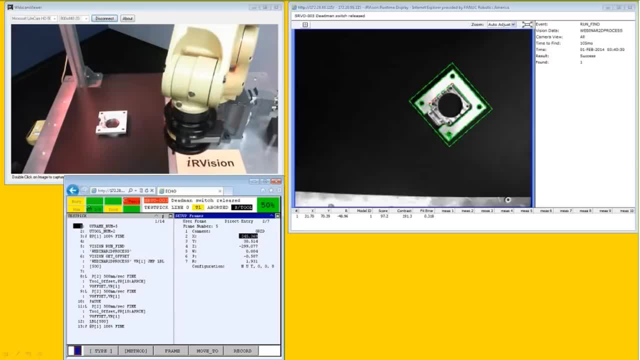 TCP for your pointer, when you train the grid frame. so let's just put some bad numbers in here, some some odd numbers in here. I'll try 340, and Let's just say 30 instead of 38. Now, how do we, how do we reconcile this? so here, here was where we add. 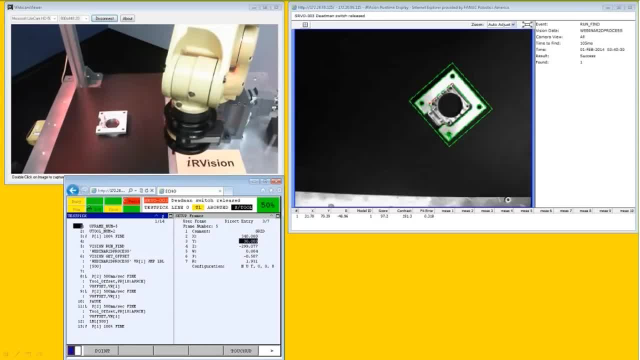 In real life. here's where we're at in real life. You have just trained your grid frame and you've trained it wrong. You've done something slightly wrong with that, with that grid frame. Let's say: we're, we think we're doing fine and we go through to our, our. 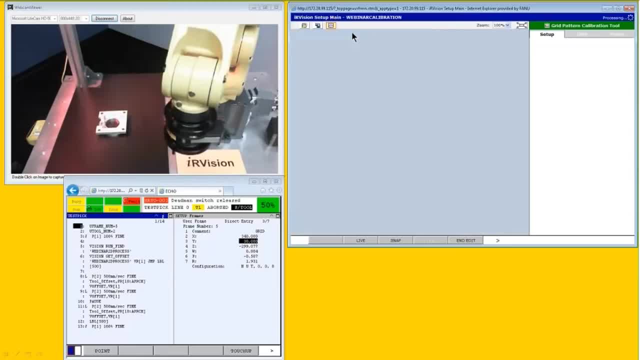 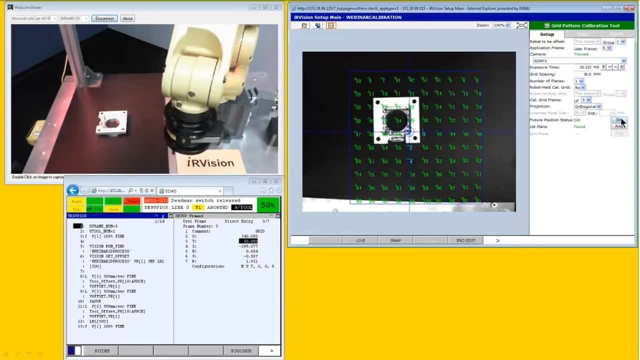 calibration process. We get to this calibration edit and we go ahead and set that user frame. I'm not going to redo my calibration again- I don't like to take time to do all of this- but I'm going to reset the calibration frame to the wrong. 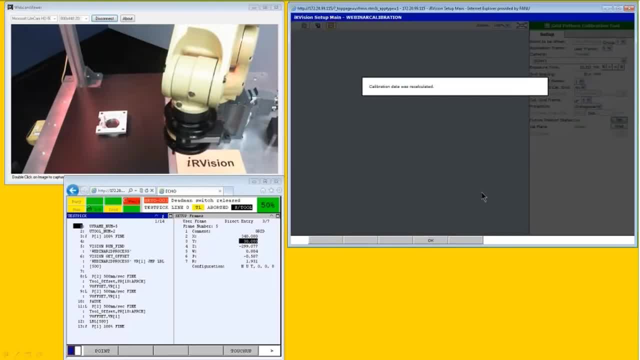 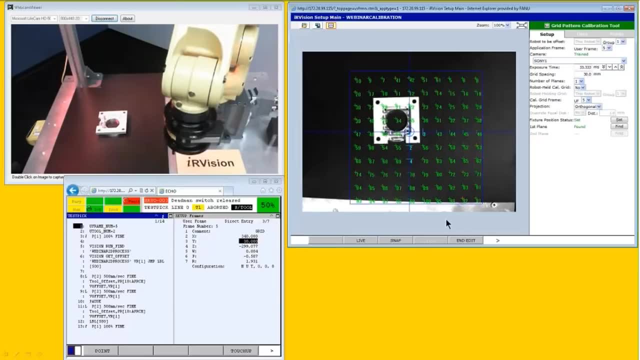 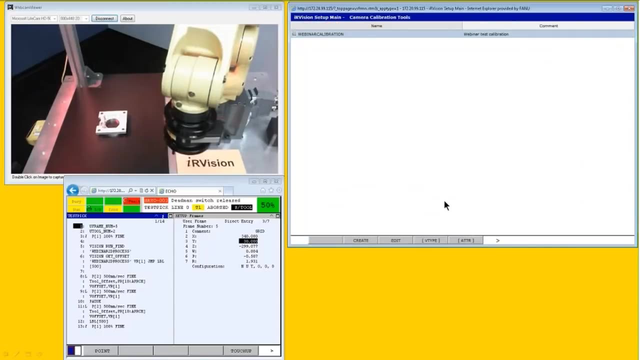 Grid by saying fixture, position, set again. This is something you'd be, these are the steps you'd be taking in real life but you, unbeknownst to yourself, you've miss trained the Miss trained the calibration Grid. we'll get out of that and go to again this, again following some of the steps. 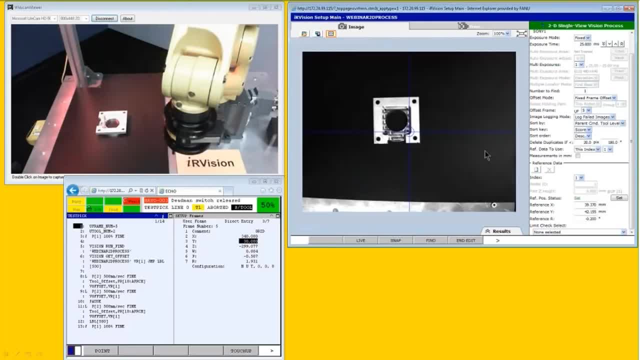 We would normally take. we'll get out of that and go to our normal. what we might normally do will position our part in space, just like we were going to train it. we already have our, our Location, the tool trained, so we might snap, find that part, think everything is fine and go over here and set our reference data. 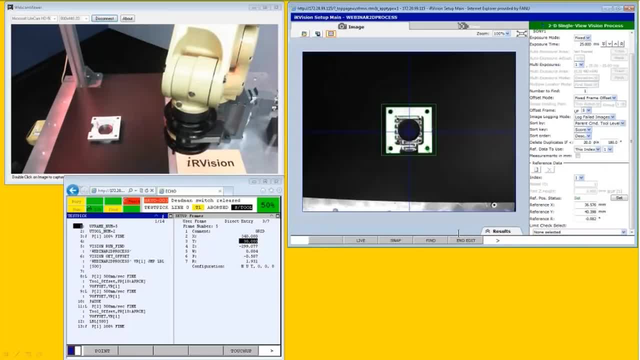 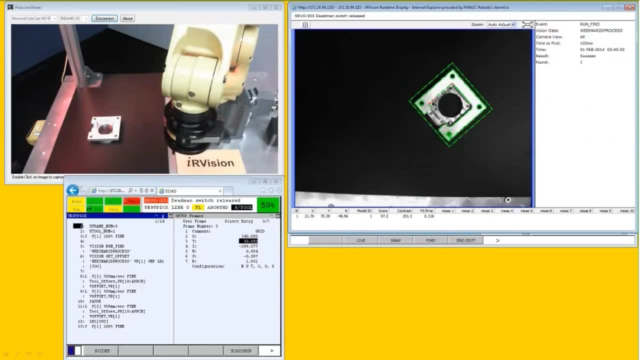 So far, so good. it complains because I've already done it. but we'll set our reference data, save that And Go to our Teach pendant program and, just like we did before, let's touch up our. let's touch up our Pick position. I'll go back to step mode. 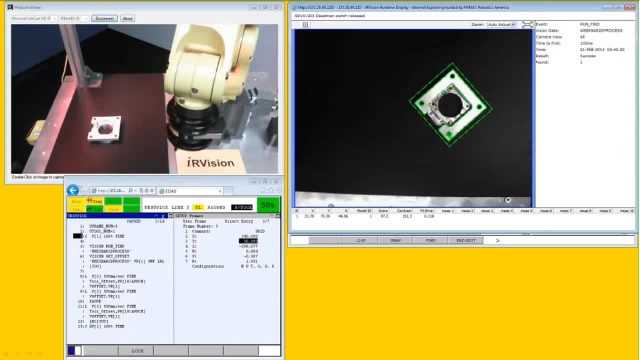 Robots at its Offset, that it's out of view position. We're going to run to find there. We go it. but I found it great. We think everything's okay. It got an offset. That's great things that we think everything's okay. 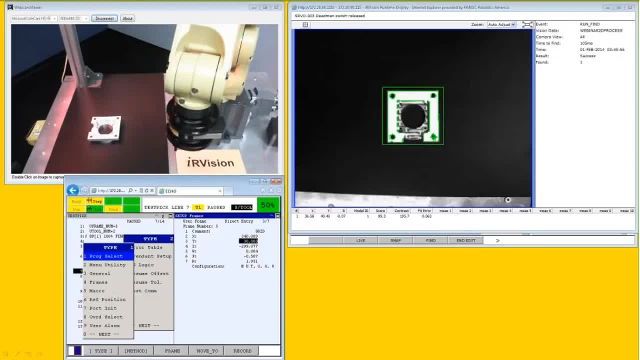 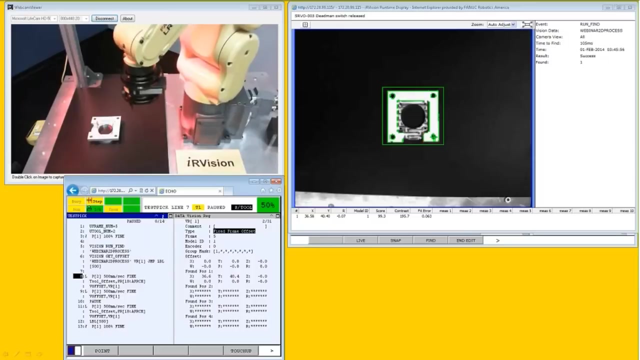 In fact, we'll go over here and look at that offset And it, the Offset, even returned all zero. so we think that's okay too. Continuing on to our point. Continuing on to our point, we will- let's Touch that point up again. you, you, you. 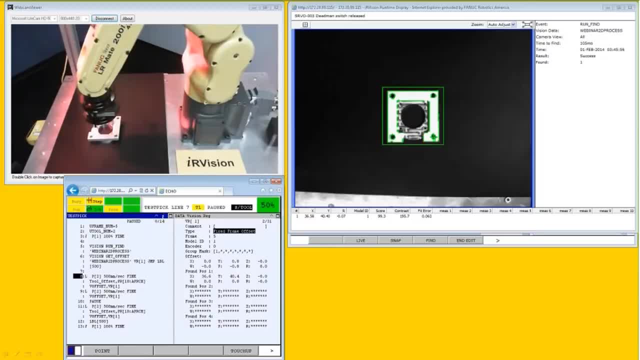 you, you. this is very typical of what happens in real life When you have done the grid frame incorrectly but you think it looks okay. So I've got the point trained again, Let's do our touch-up. I I don't want to set a new ID. 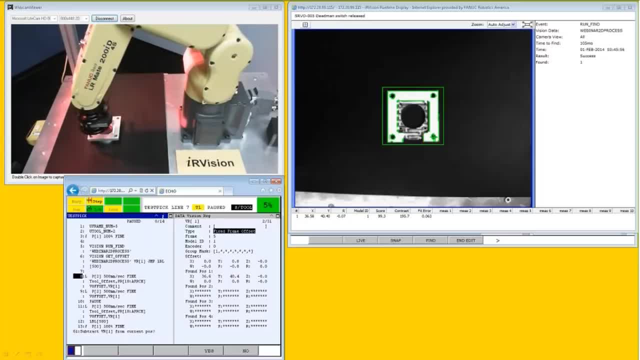 I don't again that we see zeros there, So I'm not going to subtract vision. a register from the position track. the tool offset data, of course. so now we have a taught position. let's go back to the start of our program and try that, that once. 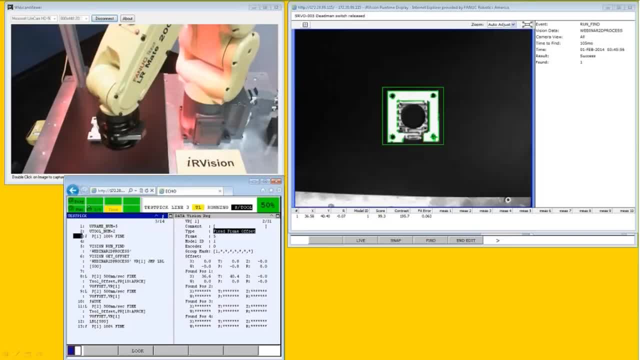 we won't move the part this time. we'll see what happens. there we go, finds it correctly, because we've just trained that and and surprisingly, not so, for maybe not surprisingly and talk about the math, but what does happen is if we just apply x and y coordinate offsets. 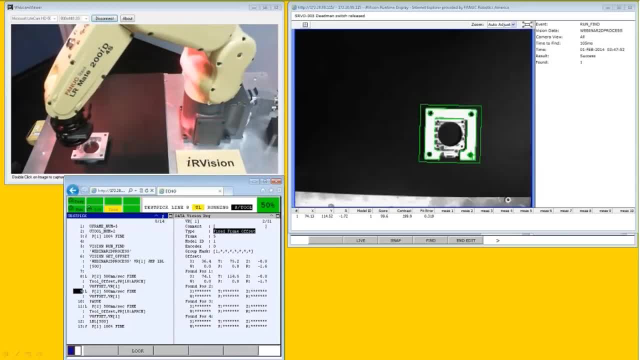 it's going to find it correctly again. here's where the thing really has problems, because our translation is no longer correct and our transformation is off by a certain number of points when we rotate the part. this is where we see the error in our grid offset. see how that no no longer finds the part. 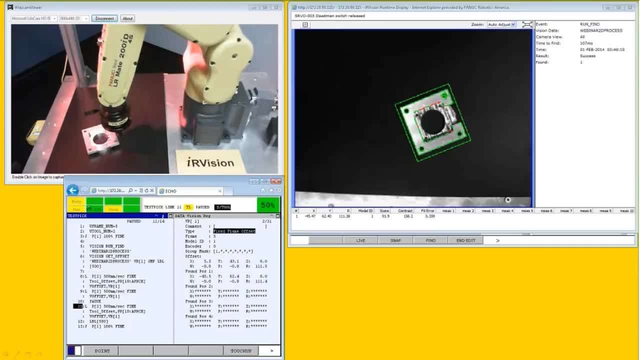 correctly. so there is a, there is a way to approach this. it's a. first of all, the way to the way to recognize this error is by what I've just done, and I think it's important. that step is important to understand that you have an error and 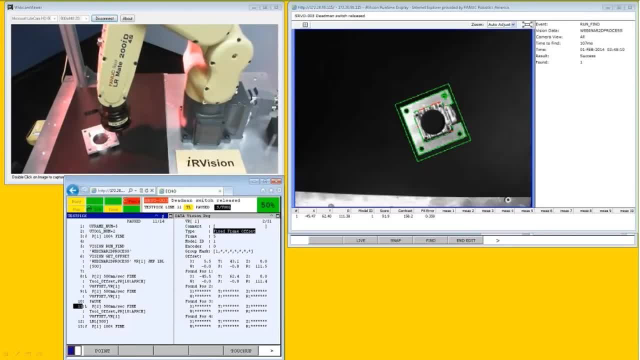 the way you first recognize the error is maybe not when you see the, the Cartesian offset and X and Y, but it might be only when you start to try to rotate the part you see the error in the transformation. so I want to point that out to you. 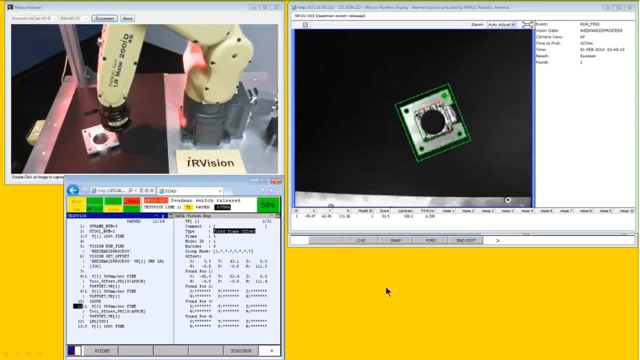 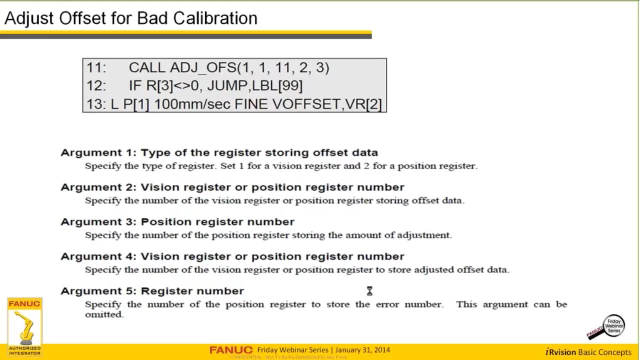 point that out to you as a common error that happens in the 2d vision process and the way to fix it. well, what I usually do when I make that mistake is: I'll go back to my grid process, make sure I've done everything correctly, trained by tool frame. 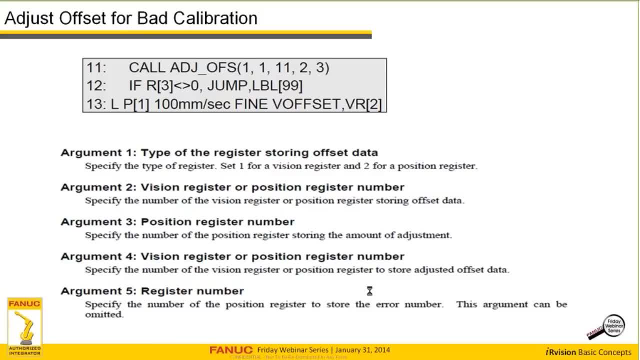 correctly, train my pointer tool frame correctly, train my grid frame correctly and repeat the process. however, should you have a bad calibration or a bad or some sort of error in your, in your system, in your, in the grid frame offset and you're not in a position to 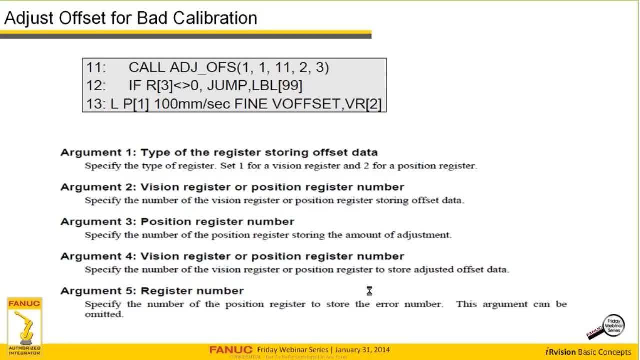 make that change, to make those to make that change, there is a quick way to make a slight adjustment that's going to fix the transformation for you and that's a Carol program called adjust offset. the way that just offset works is it takes the. you can specify either a vision, 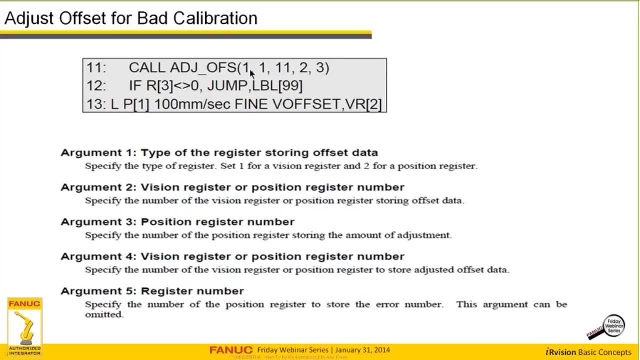 register or a position register? who will specify our vision register? it takes the vision register that we just received as an offset. it applies it against another arbitrary register, storing the amount of offset, and retains it to us in a new register, a new vision register. then we use this new. 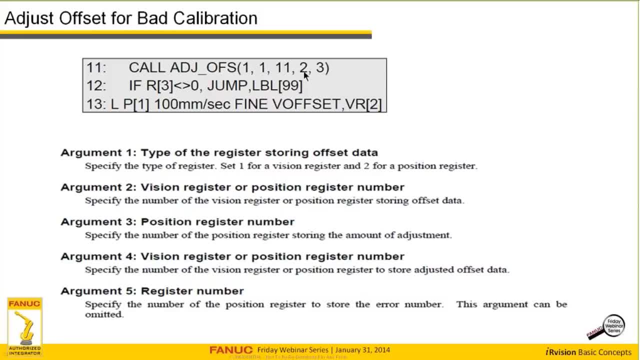 vision register instead of the old vision register to for our vision register offset. the result of this Carol program is then put in register 3.. If it's not zero, it has not succeeded at transforming the offset. We won't go into this process right now, but I want to point out to you that this is a useful 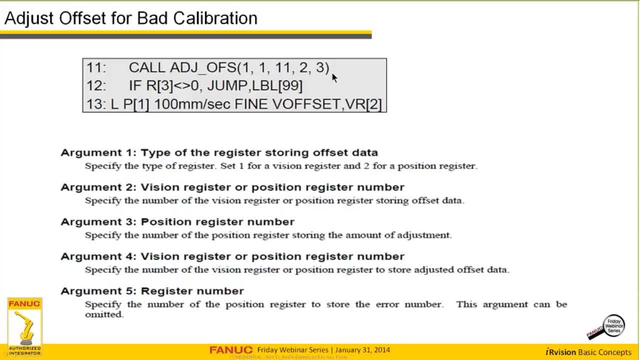 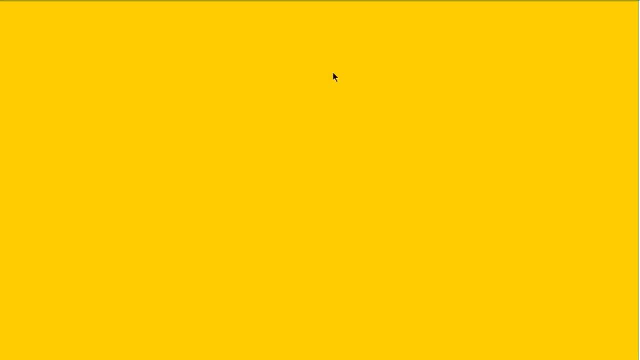 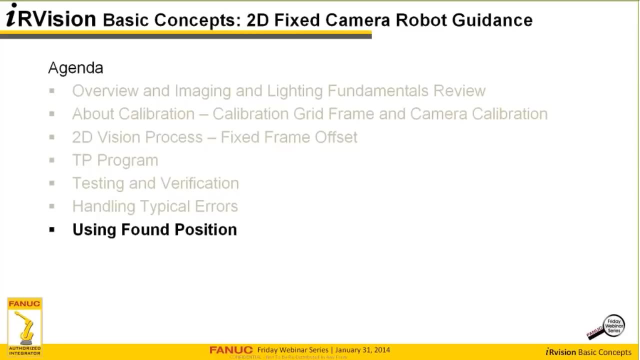 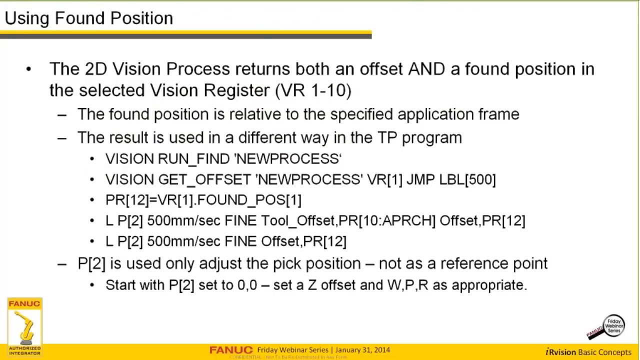 way to manipulate your, to manipulate your. an error, a minor error in your calibration. Finally, one last word about another way you can use the vision system, the 2D vision process, by not using the offset but by using the found position. You may note in your teach. 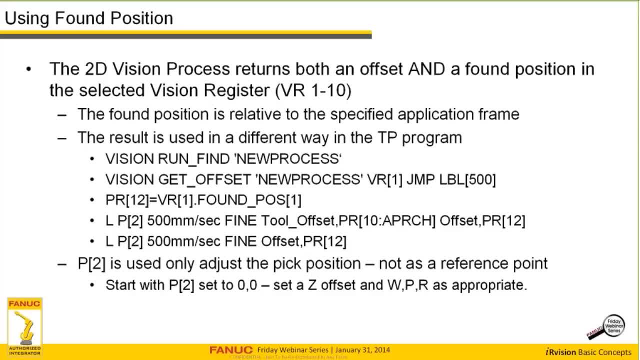 pendant, under looking at vision data, that the 2D vision process returns both an offset and a found position, and both of those are contained in the selected vision register. That'd be the vision register, one to ten, that you've selected in your TP program, The. 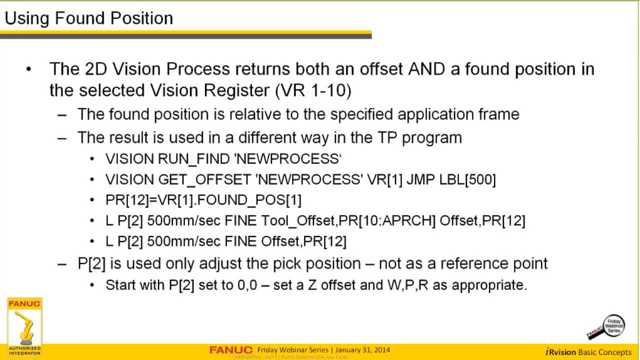 offset and the found position are both contained in the selected vision register. The offset position we've already defined. The found position is a little. it's pretty easy to understand. It's a position that's relative to. it's a real world position that's relative. 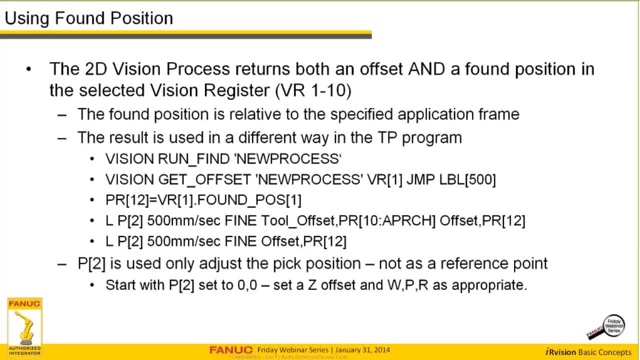 to the specified application frame. So if the part is at zero, zero if it's at, if it's at its reference set point, if it's at the- excuse me- if it's, if the origin of the part's at the zero, zero point of the frame, the found position will be zero. If it's ten millimeters. 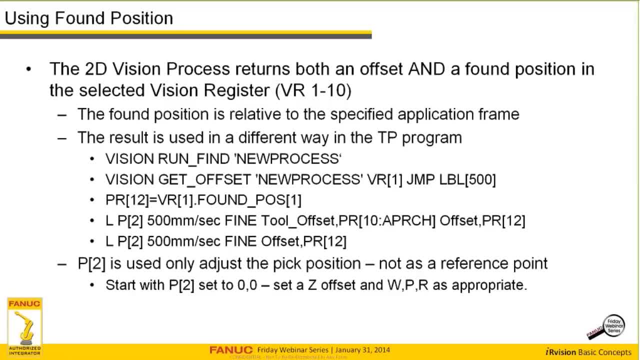 x and y from the frame, the position will be x and y plus ten. You use it in a different way in the TP program, however. You still run a find and you still do a get offset. However, we will take the found position of that vision register and place it in a temporary. 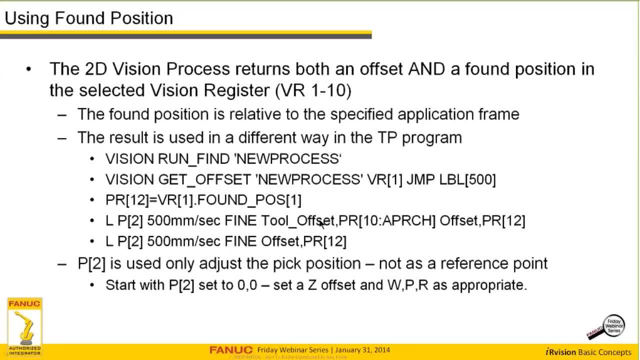 position register. From there we'll still use our tool offset, our tool offset for an approach point, but we'll use the position register as a standard offset to a known point, both for approach and for pick. The thing that's different here is that the position